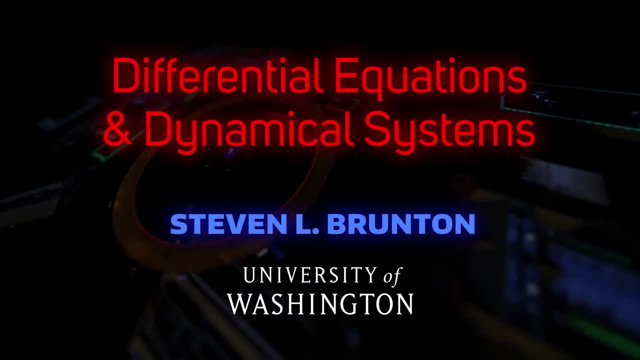 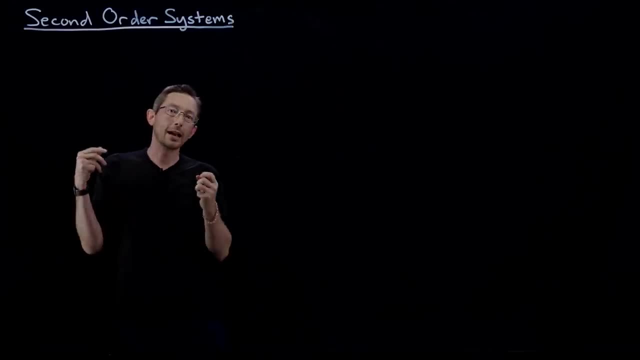 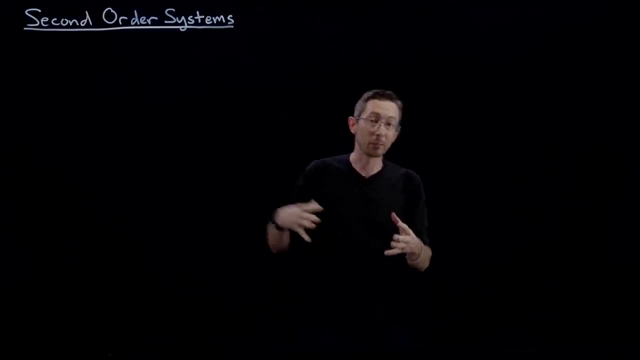 Welcome back. So in the last few lectures we have derived from scratch simple first-order linear differential equations, and today we're going to take a pretty big step, going from first-order differential equations where you only have a single derivative- dx, dt- to second-order differential equations where you have second derivatives- d, squared, x, dt and things like that. 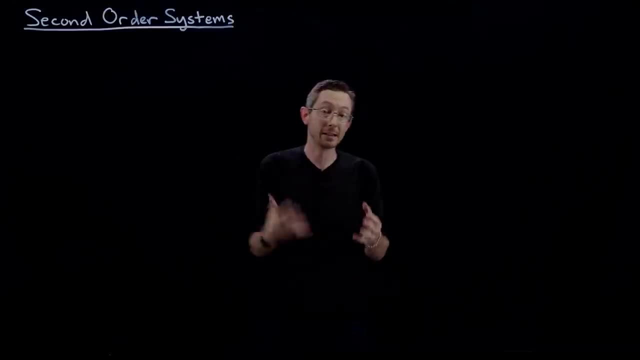 And these systems are going to come up all the time in physics because Newton's second law- f equals ma- is in fact a second-order differential equation. Okay, so I'm just going to start by a simple example, by kind of writing down a simple example from physics where we can write down: f equals ma and then we're going to see how to solve that second-order differential equation. 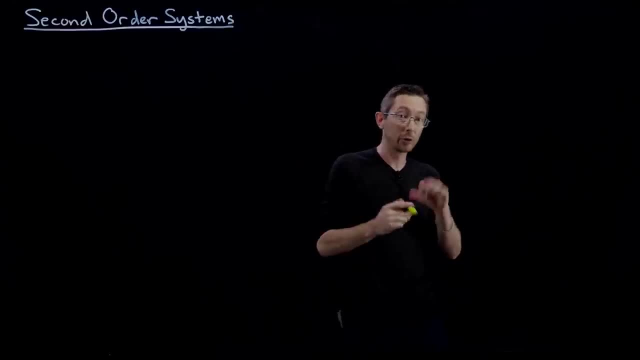 Good, And I think I'm going to solve it four ways. So we'll have, you know, four different ways to solve the second-order linear system. So the system I want to look at is called the harmonic oscillator. harmonic oscillator, And that is just a super fancy term. You've heard harmonic oscillator before, probably. 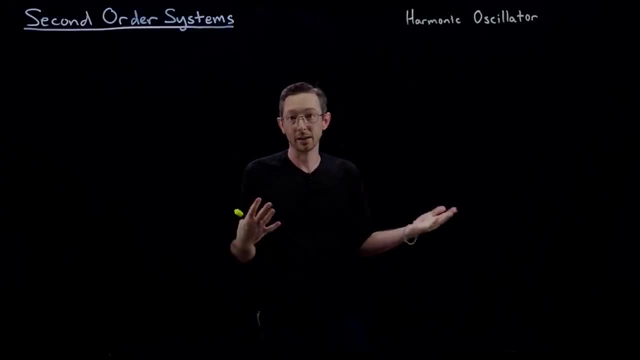 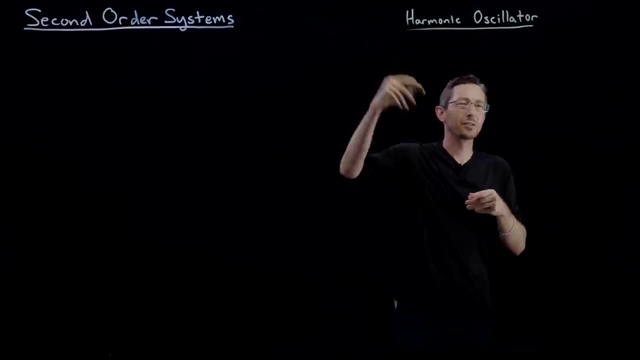 It's just a really, really fancy term for anything that oscillates linearly, Like if I have a mass on a spring or if I have a pendulum. those are both examples of harmonic oscillators. These also come up in optics and quantum mechanics- all over the place. 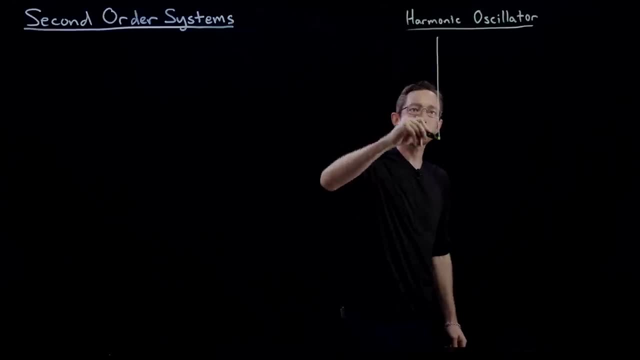 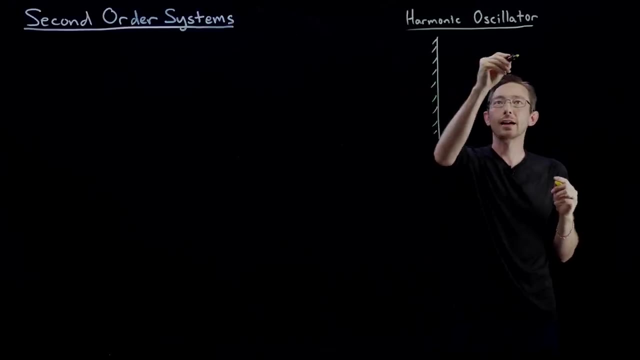 You know electromagnetism, So the example I want to draw is where you basically have. I'm going to draw this horizontally because I don't want to consider gravity. Just imagine that I have a mass, a mass m, attached to a spring, with a spring constant k. 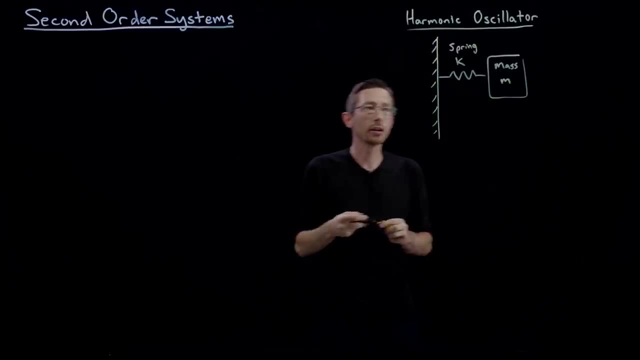 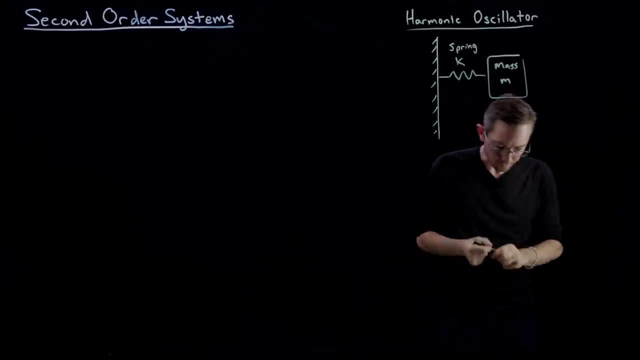 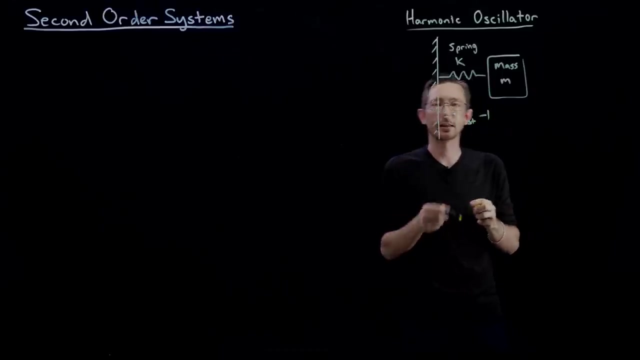 Okay, so this is a spring And we're going to assume that it has a rest position. So there's basically a rest position for the spring k Where basically, you know, there's some x rest. that's this length and anything in addition. so the center of mass, of this, of this mass from that rest position is going to be called my variable x. 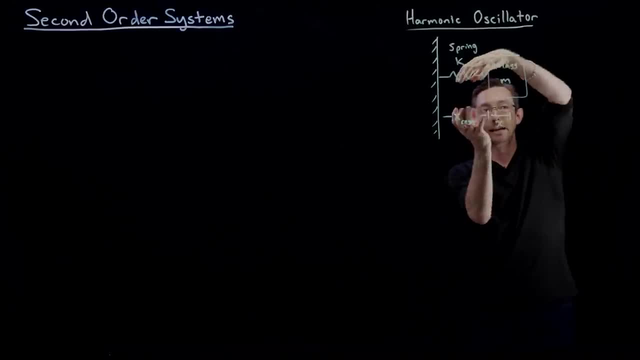 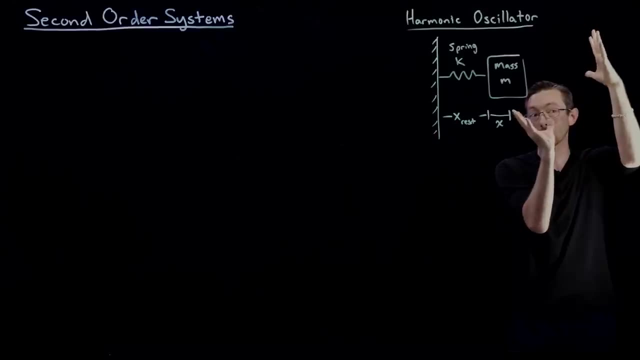 So the state of the system that we're going to model x as a function of t is basically the position of this mass away from its rest position. So I'm going to do things like I'm going to pull this mass away from its equilibrium and let it go. 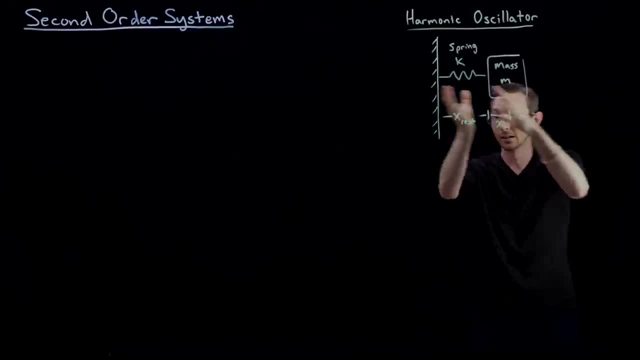 And you're going to, of course, in your mind, see this thing oscillating: x of t is going to give me sines and cosines. probably That's what we're going to model, And we're going to start with Newton's second law. 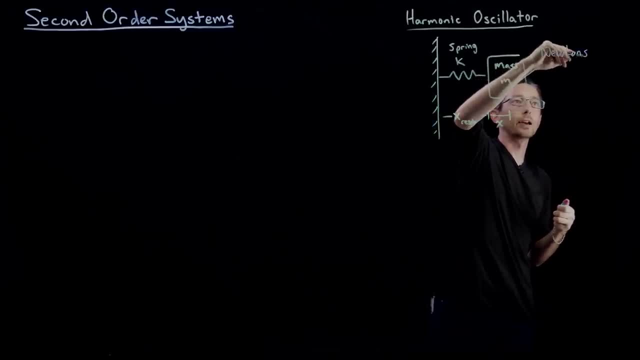 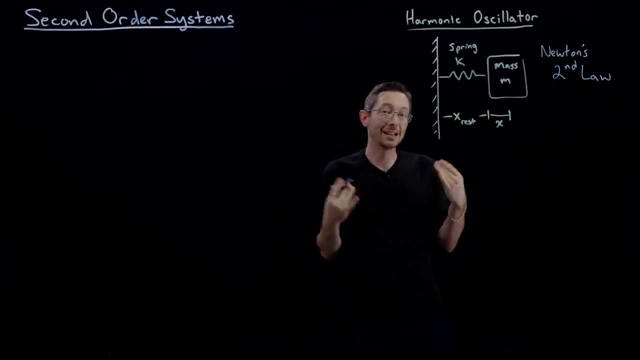 Like I said, we're going to start with Newton's. this is a brand new, very nice pen. Newton's second law of motion, which you all are familiar with, as f equals ma force, equals mass times, acceleration, And of course acceleration in this case is: 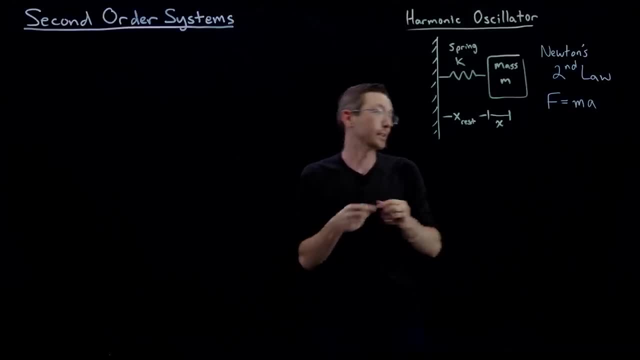 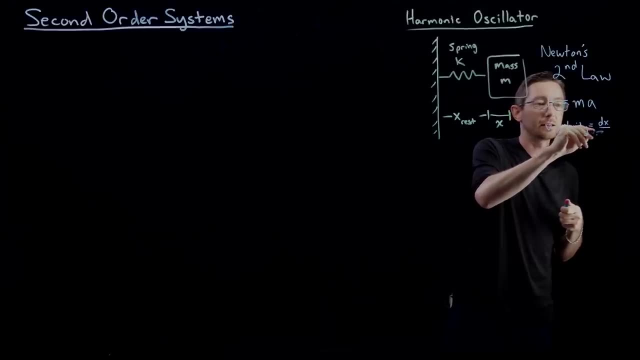 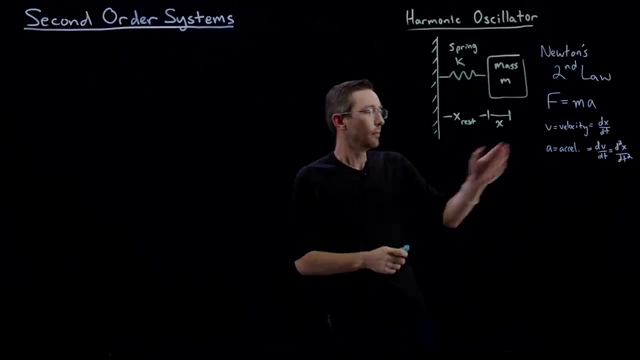 is the second time derivative of position. So velocity, let's just say, you know, v equals velocity, equals dx dt. a equals acceleration, equals dv dt, which equals d squared, x, dt squared. Sorry if that's a little small, but this is. you know, what we're all familiar with from basic, basic physics is that you know x. 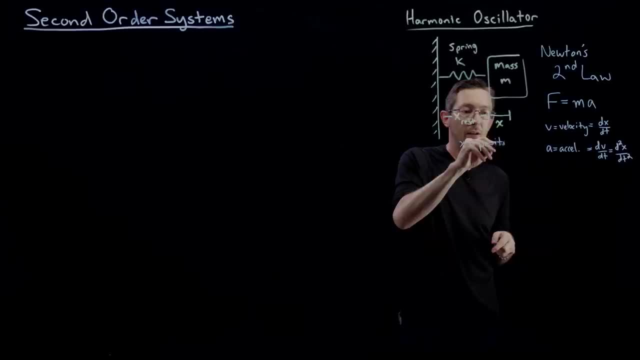 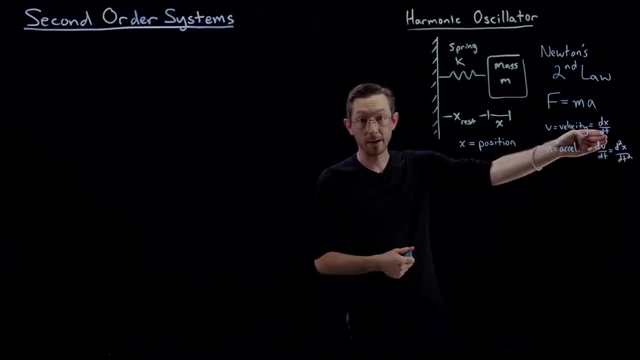 it is my position of this mass away from equilibrium. v is the velocity, a is acceleration. so the velocity is the first derivative of my position in time, the acceleration is my second derivative of my position in time. And this is where that second order is going to come from. is now we're going to have a second derivative. in x we're going to have a differential equation in terms of the second derivative. 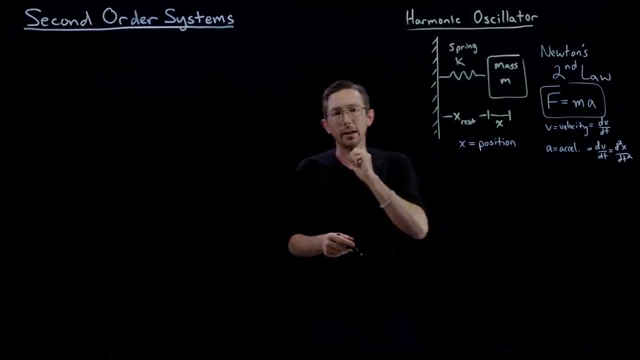 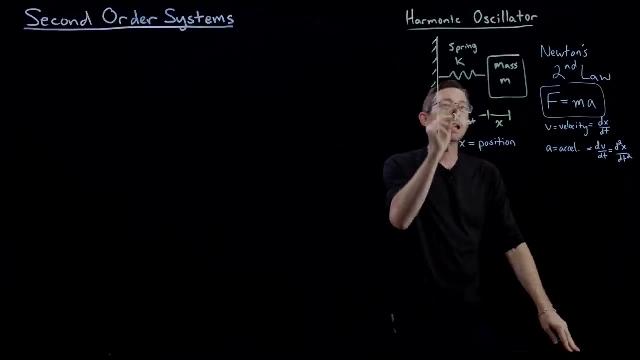 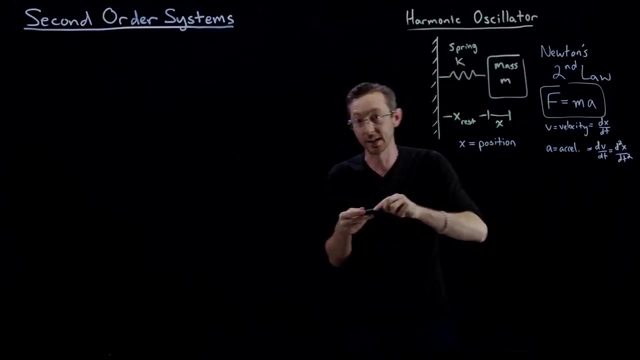 In fact this is Newton's second law. So how do we derive this? We say, you know, x is dx The displacement from its rest position, and the force on this mass is proportional to k times x. So this is just again. this is- I think this is Hooke's law or something like that- where you know, the more I pull this mass away from its equilibrium, the larger x is, the larger the restorative force from that spring. 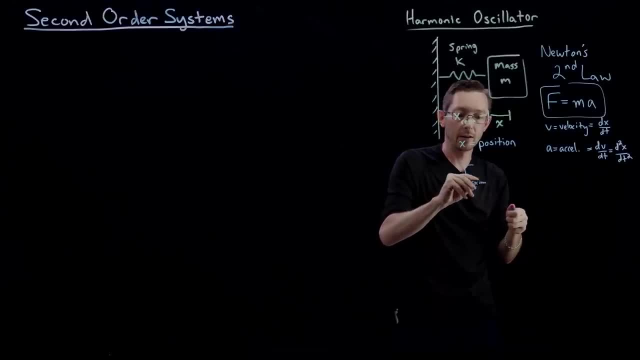 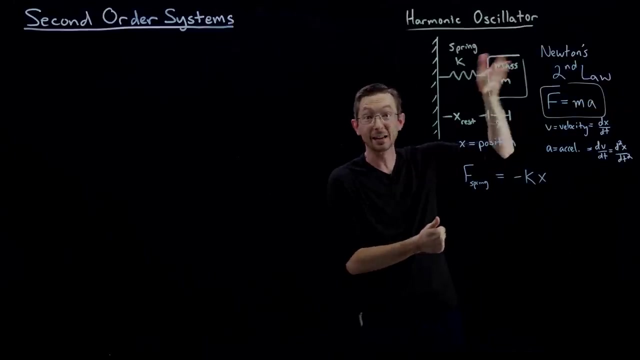 So the force from the spring, the spring force is, I believe, going to be minus k times x. So if I pull x in the positive direction here, I'm going to have a restoring force trying to pull it back, you know, in the negative x direction. 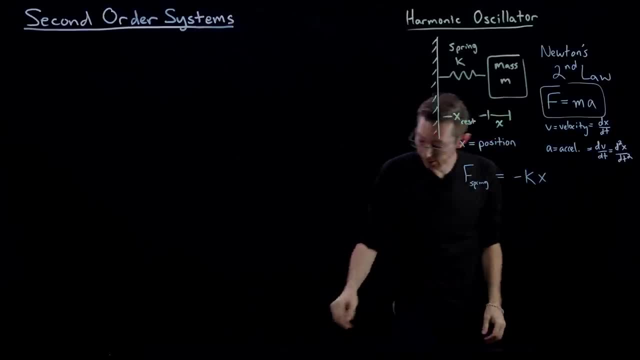 And it's going to be proportional to x. OK, so this is actually really really easy. I think the first thing I'm going to do is you know we're going to start by assuming you know mass equals one and k equals one. 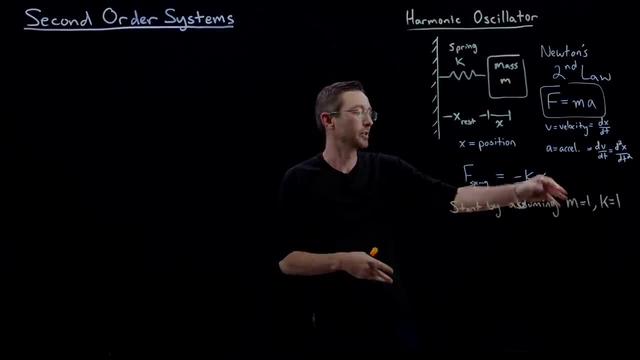 We'll relax that a little bit later, But we're just, you know, to make my life easier, i'm just going to assume that the mass is one and the spring constant is one, and so what we get when we write down newton's second law is that d? dt of um? how? 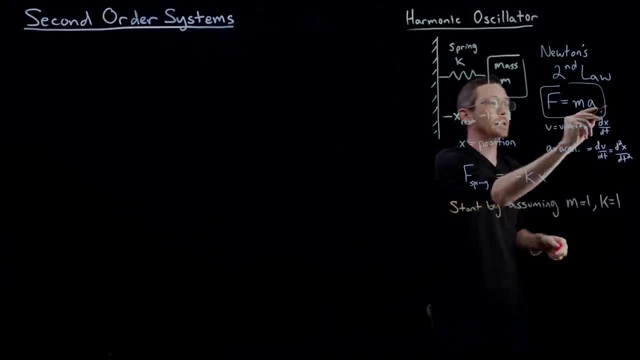 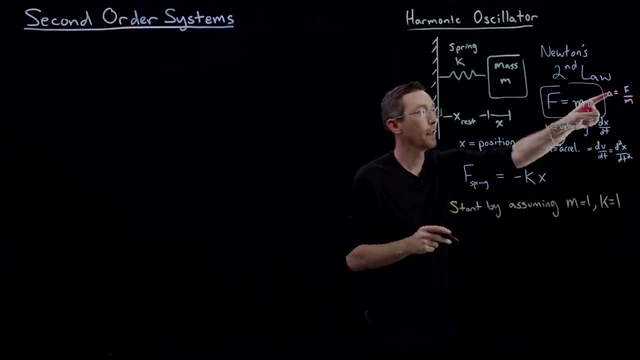 do. i want to write this so you know you can write this as a equals f over m. that's also fine, and m is one, because i said my mass is equal to one. so my acceleration is d squared x. dt squared, that's a, and that equals my force divided by one. and my force is minus. k is one. my constant is one. 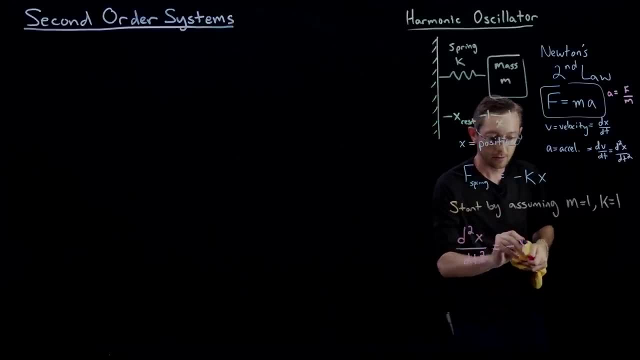 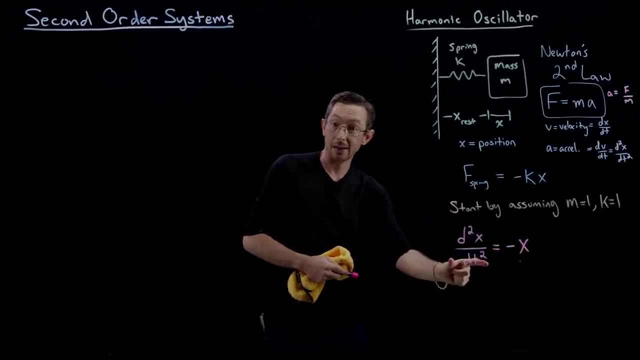 i made everything one, so it's just minus x. that's my differential equation. this is literally newton's second law: f equals m times a okay. force equals mass times. acceleration mass is one, my spring constant is one, so i get x. double dot equals minus x. and yeah, if i want to write this in a little bit, 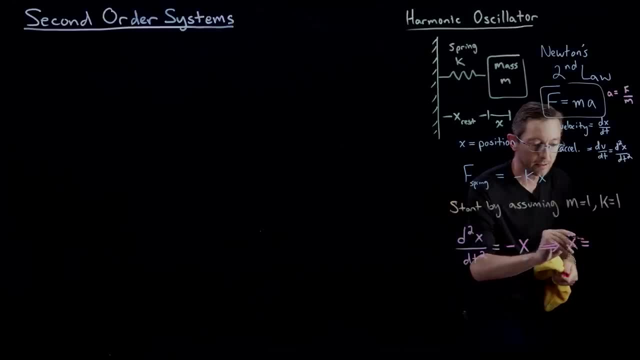 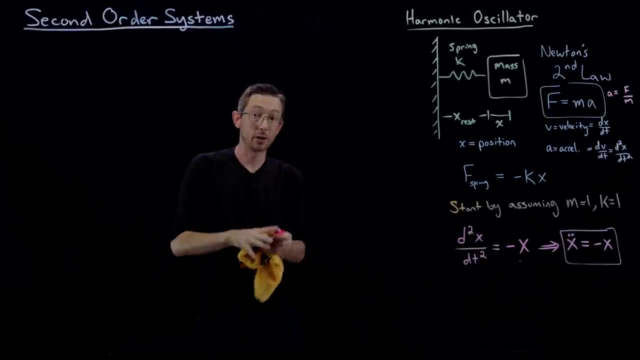 simpler notation, i'll just say x double dot equals minus x. this is my simplest second order linear differential equation. this comes up all the time in physics. pretty much any system that oscillates, any system that is periodic and linear, like a pendulum with a small angle, or this mass on a spring. 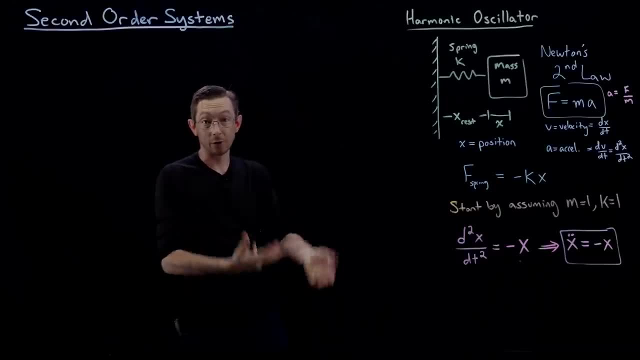 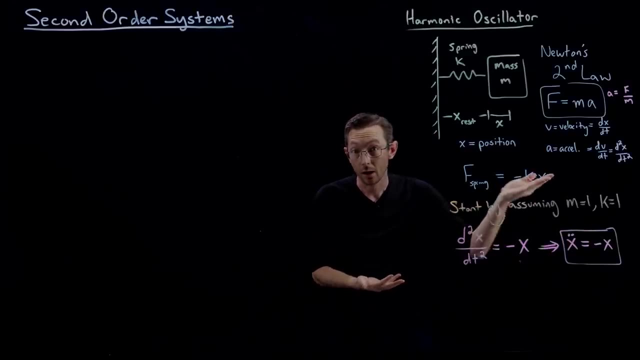 you know, lots of phenomena in optics and electromagnetism and quantum mechanics are also oscillatory and linear, are going to be governed by this second order linear differential equation that we call the harmonic oscillator equation. okay, so we derived it from first principles. f equals m, a is generally. 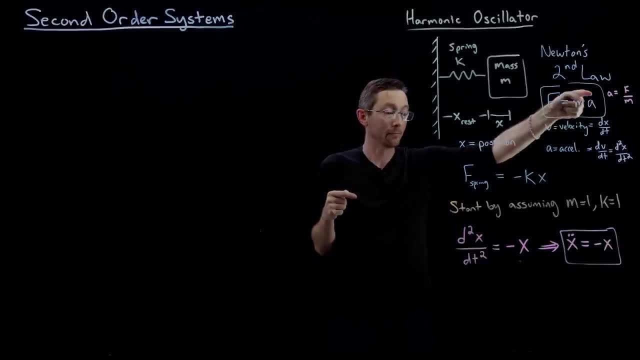 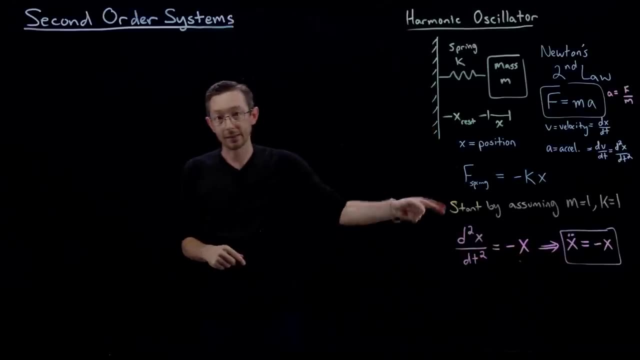 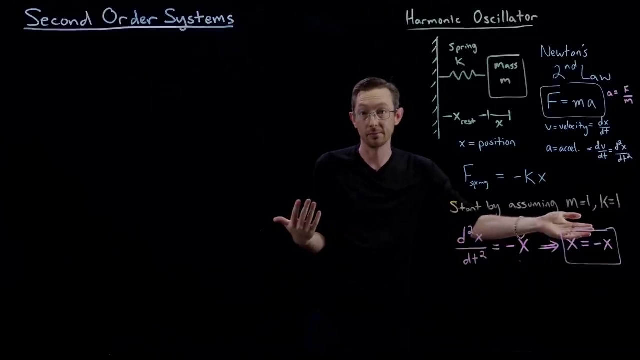 speaking, going to give us second order systems because a is the second derivative of my position or my state. good, so now we're going to solve this differential equation four ways and i'm going to build up a bunch of lectures on you know kind of how to understand these second order systems. good, 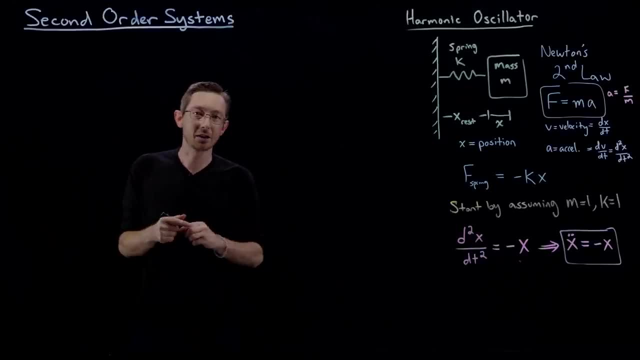 um, i kind of, uh, i like to start with the easiest approach, so so method one, uh, method one, and this is second order systems, literally x double dot equals minus x, in case i erase this. so method one is is pretty simple, um, and i actually find this to be a pretty useful. 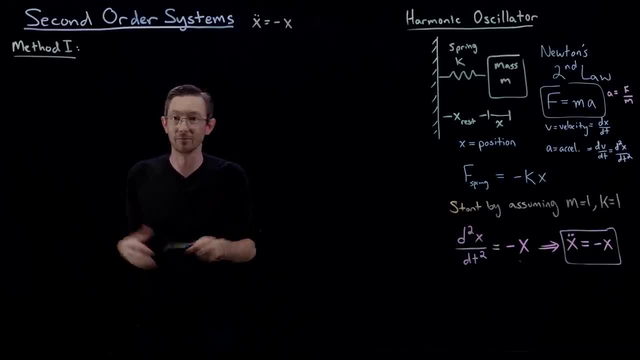 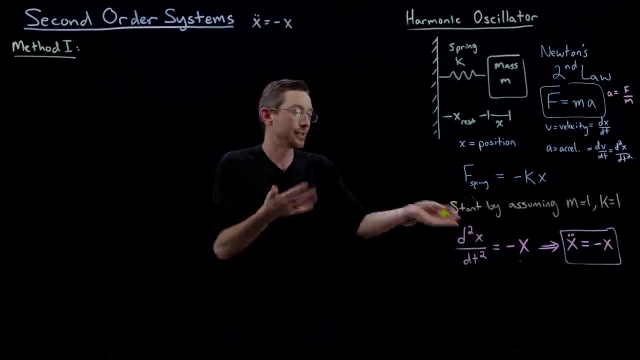 approach in differential equations- this is what people have done for for centuries- is you guess what the solution is and you plug it in and you see if it works, and you see if it doesn't work. and it works. it's like actually very physical. this is what we call the physics solution. this is what i 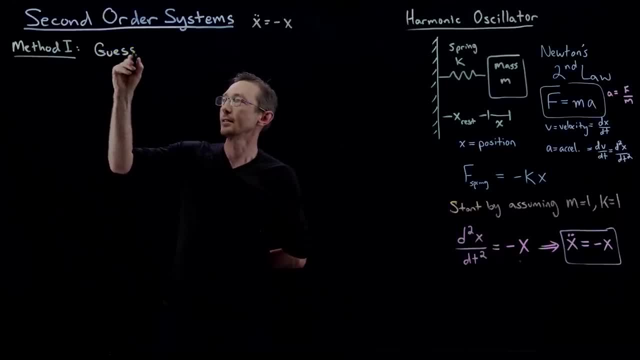 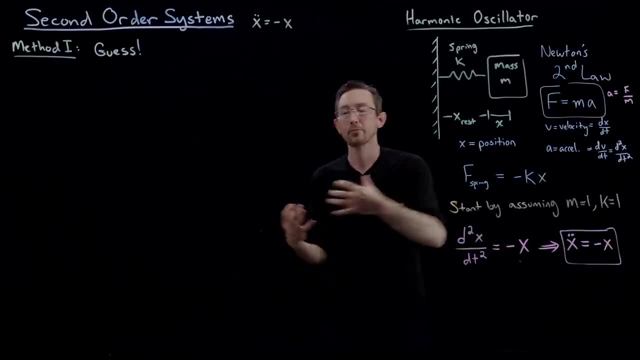 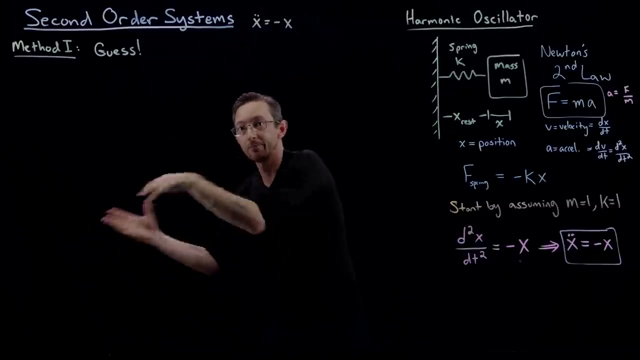 call the physics solution method. one is guess. okay, so guess, and what's a pretty good guess for the function x of t? okay, so we know that if i pull this mass, i guess it's over here. but imagine, you know, i'm pulling this mass and i let it go and it starts oscillating. what is a function? 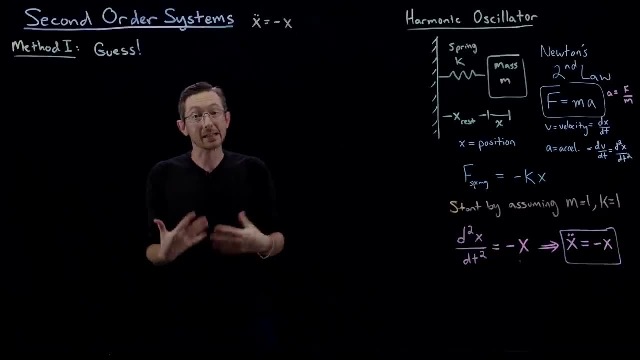 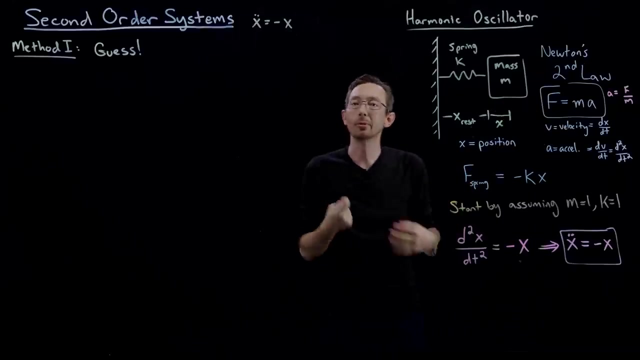 that oscillates in time. well, our basic functions that oscillate in time are cosines and sines. okay, and at t equals zero, sine of t is zero. so if i have a non-zero initial condition, i'm probably going to get something that looks a lot like a cosine function. okay, because it's going to. 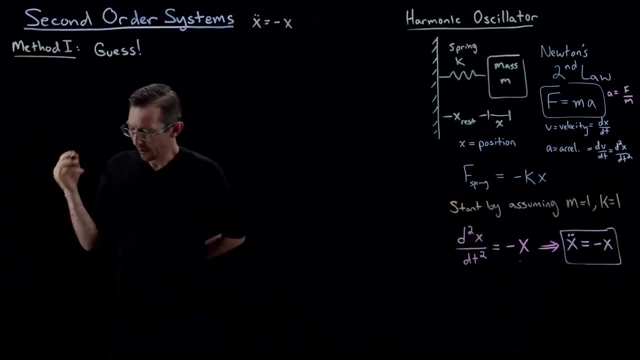 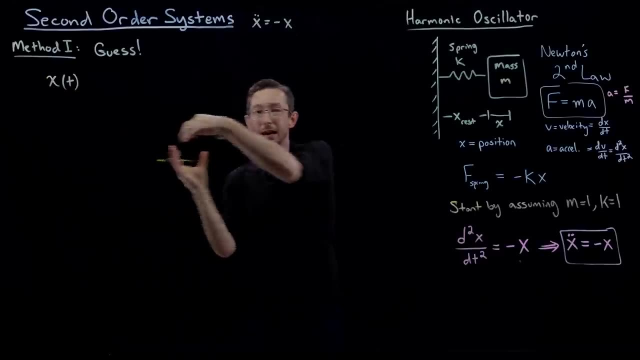 oscillate and it starts off not at zero. so i'm going to assume that my uh, my system, x at t the position of this thing when i, you know, at time zero and it's going to have some initial condition, let's say um, x at t. so i'm going to assume that my uh, my system, x at t the position of this thing. 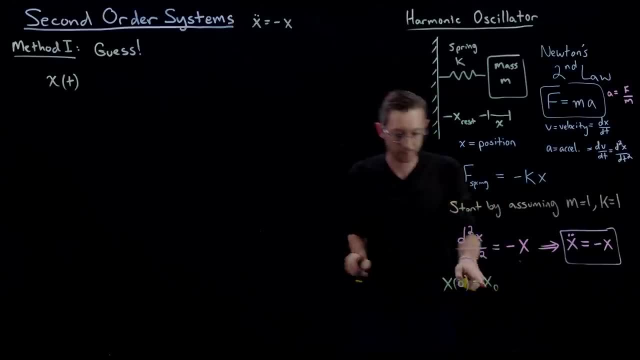 at time zero equals x naught. okay, it's some non-zero initial condition, and maybe i'll say my derivative x dot: at time zero equals v naught. let's say that that equals zero. so i start this thing at an initial position, but with no velocity, and then i let it go. that's what this says. is that? 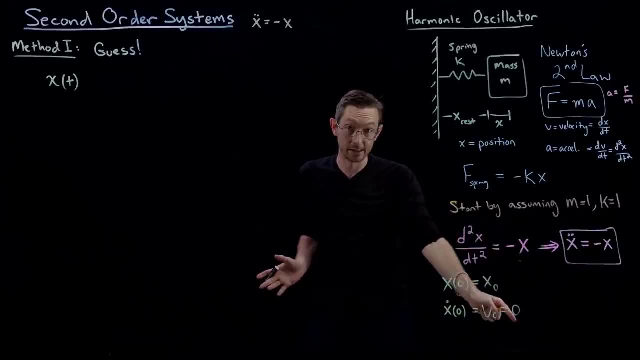 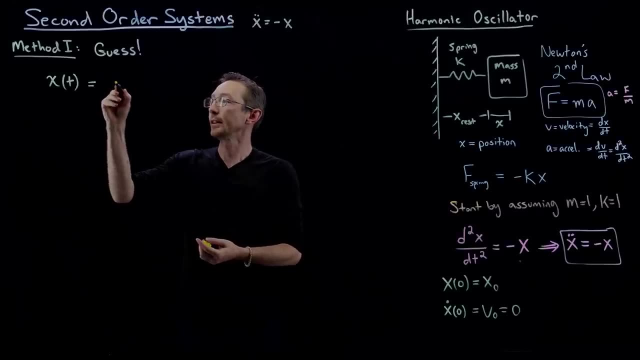 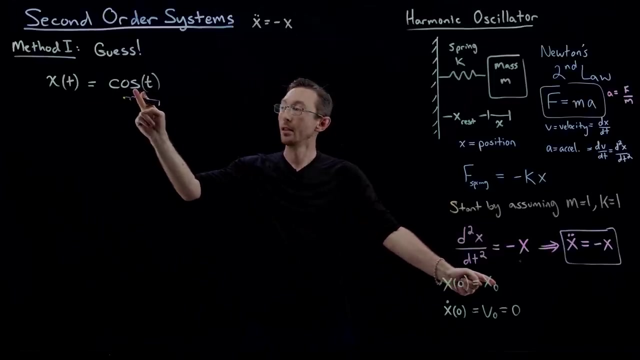 the initial condition is x naught and my initial velocity is zero, then a very reasonable guess would be sines and cosines for this function, x of t. and specifically i'm going to guess that it is a cosine function because at t zero, cosine is non-zero and at t zero, the derivative. 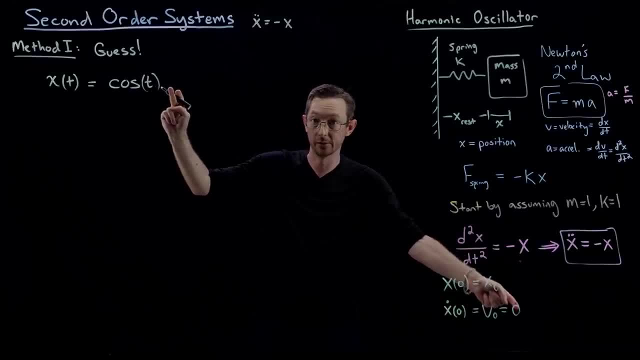 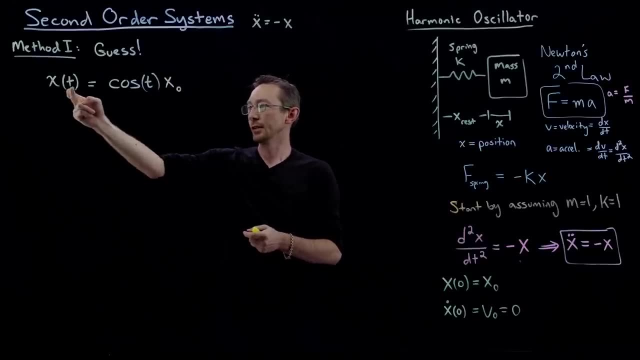 of cosine is zero, so this matches my initial position- zero velocity- and i'll need to multiply this by x- zero, okay, so at time, zero, if i plug in zero, for time x naught equals my initial condition. so this is a very reasonable guess. okay, and this is what we do a lot in in physics and in math, and 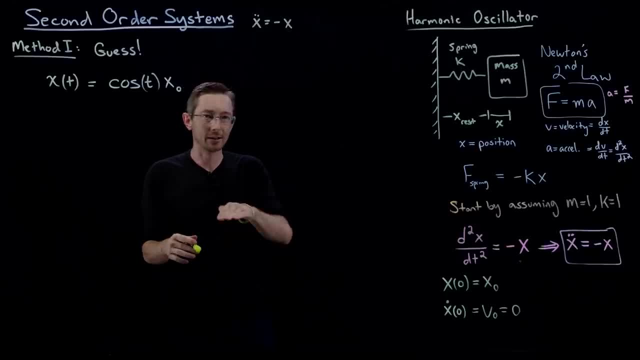 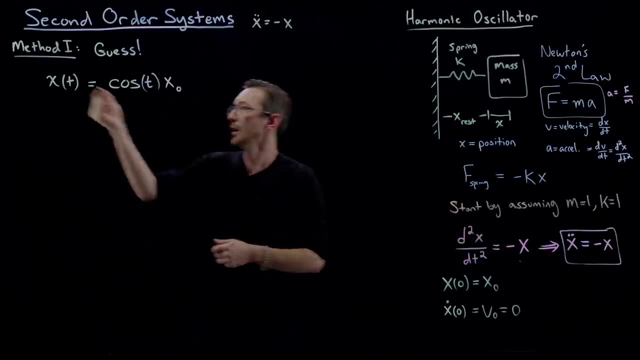 applied math is. you look at your system and you say to yourself: well, okay, this is growing exponentially, or it's decaying or it's oscillating, and you kind of get some intuition about what you think that solution is going to look like. so of course, x dot of t is going to equal minus sine of t, x naught, and then x double dot of t is again going. 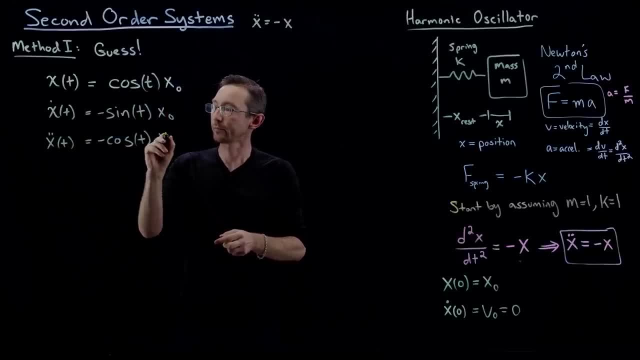 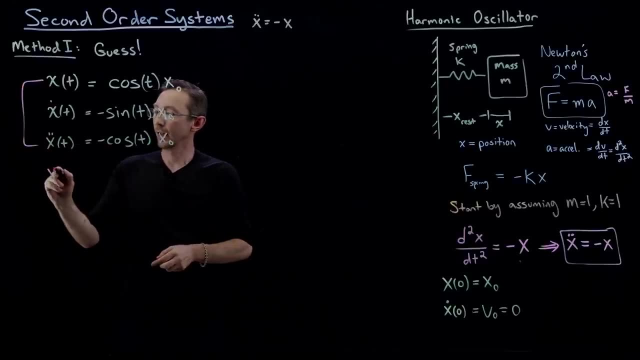 to be minus cosine of t, x naught, and you can verify. you know really simply, almost in your head that yes, in fact, x double dot is minus x of t. so these functions satisfy this differential equation relationship. that has to be true at all times to satisfy newton's second law. right, newton's second law. 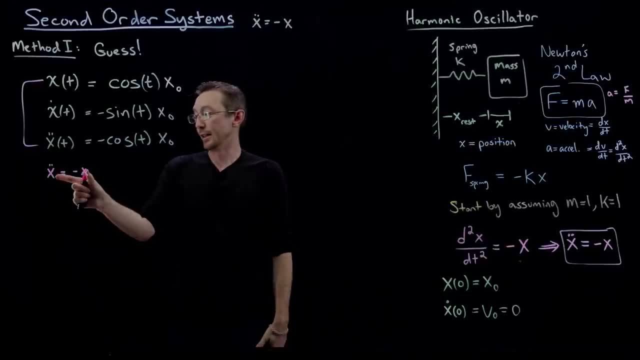 is essentially conservation of momentum. uh, and- and this is true always, it's true every you know for every system that i draw a big enough box around. this is going to be true and you can verify just by inspection that if i choose this function, cosine of t, then its second derivative, 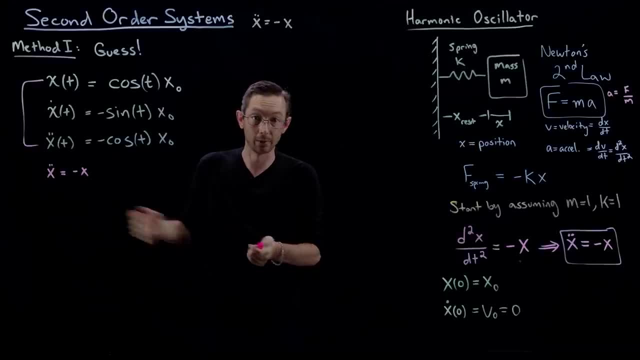 is minus sine of t, and if i choose this function cosine of t, then its second derivative is minus cosine of t and it satisfies this relationship so kind of. you know, in this case, for these linear, simple systems, we can kind of guess and we usually get the right answer. okay, good, um, and i'll just 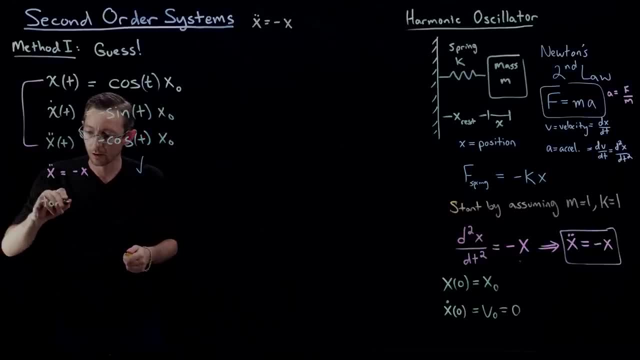 write down that, uh, you know, for general, for general, uh, mass and k. you're going to get specifically that now you know x of t equals, uh, i think, cosine of t. and then you're going to get- sorry, this is so squeaky, let's see if i can switch to this one- you're going to get cosine of root k. 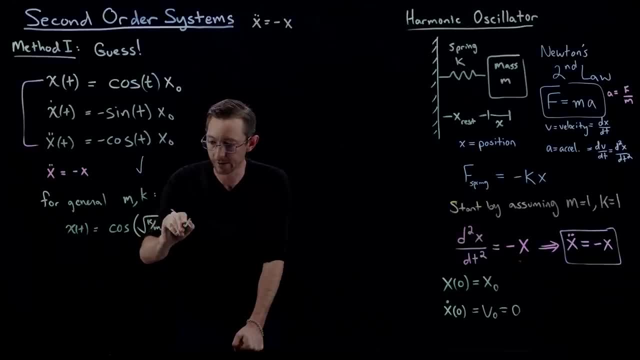 over m, t times x naught, where essentially this uh k over m square root is like the natural frequency. so you're basically going to have, like uh omega equals root, k over m is going to be the natural frequency of uh, that oscillating mass uh on a spring. okay. 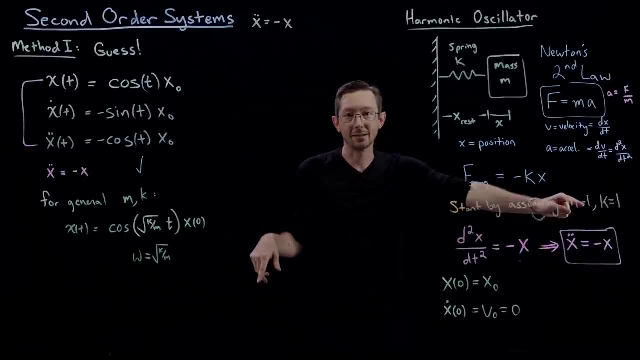 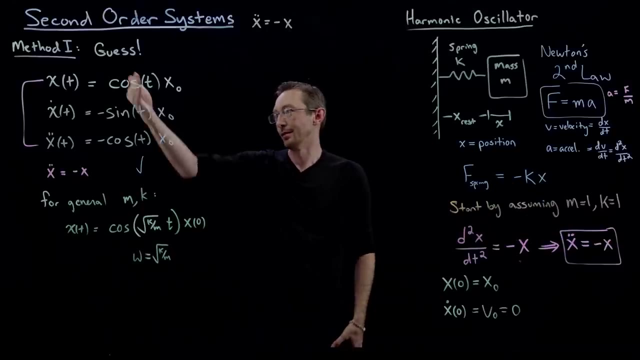 and you can derive this one from scratch. so what you would do is you would not set m and k equal to one and you would keep this as minus kx and you would keep this as m times x double dot, and then you divide both sides and you get x double dot equals minus k over m x, and you would find in fact: 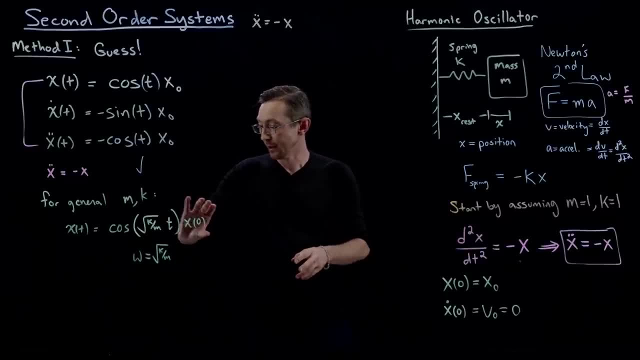 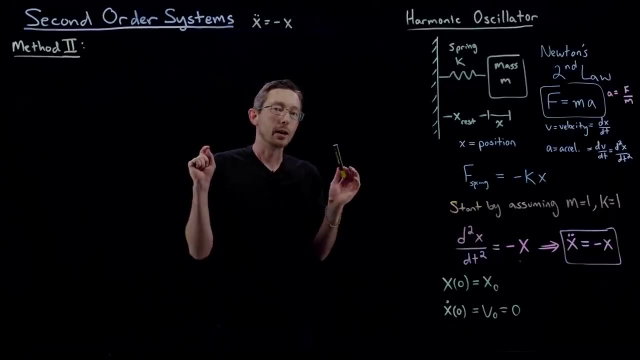 that this is the solution. so that's a homework for you- is to again, you know, verify that. if i take the second derivative of this, that equals minus this, okay, okay, um, i'm going to erase this and then we're going to try method two. okay, so, um, there's a lot of ways to skin this cat. don't skin cats. 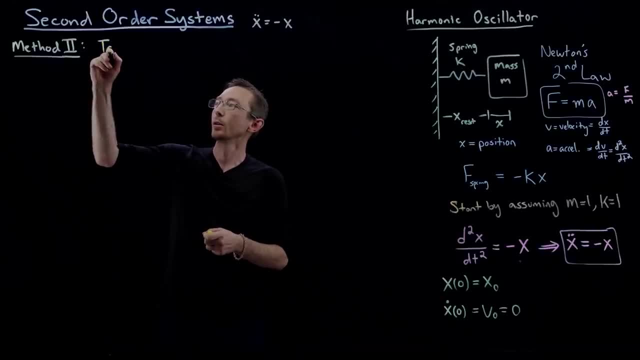 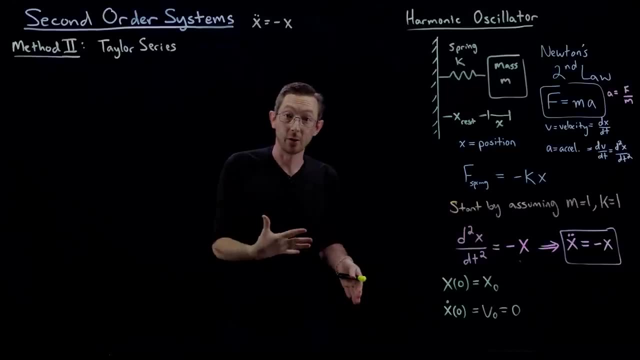 and there's a lot of ways to solve this problem. the second method uh we're going to use is the taylor series and again, i don't really recommend, you know, most of the time solving differential equations with taylor series expansions, unless you have to. but i like to show this method because 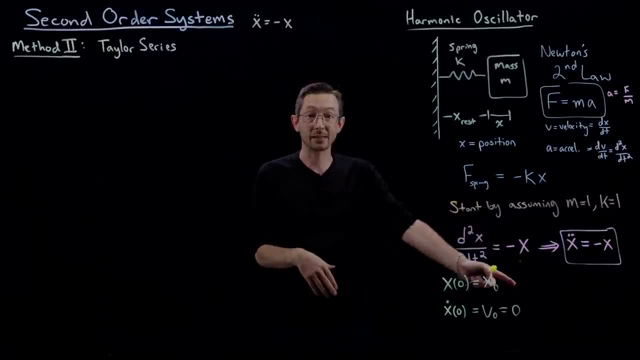 if all else fails, you can always just, you know, expand x of t and powers of t and solve for the coefficients. and it actually works, because you can solve for the coefficients and you can solve for singular constants or your exact numbers and theirpace equations in this case. so i'm going to 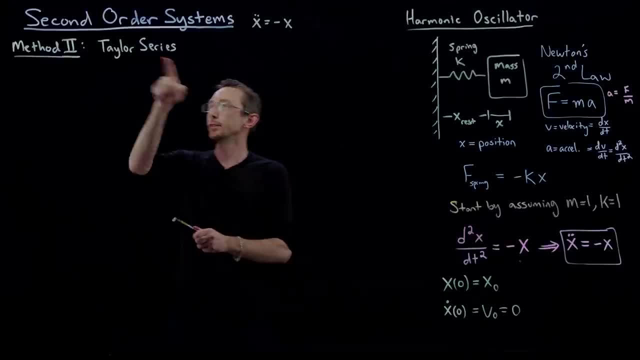 show one way to get rid of these variables. you know, supplied by apply model and actually is pretty useful at this stage just to build intuition for what's happening. so that's what we're going to do, and this is just like we did in the last few lectures. so i'm going to write down: um, where do 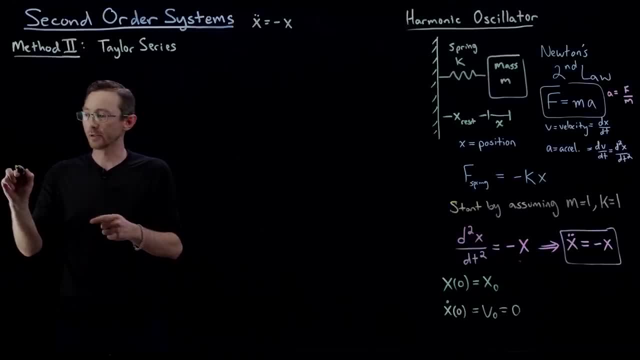 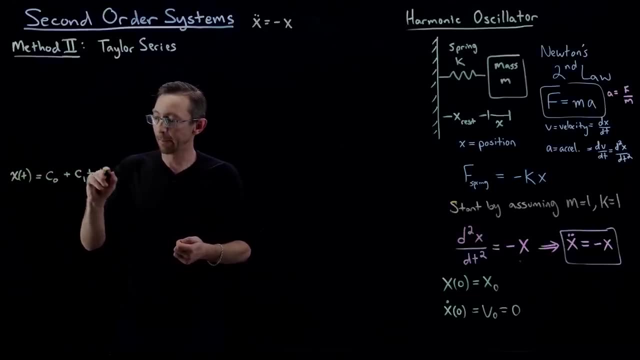 i want to do this. i probably don't want to like chop my head off. so let's say i start here and i'm just going to say: you know, x of t equals some constant c naught plus c1t plus c2t squared and: 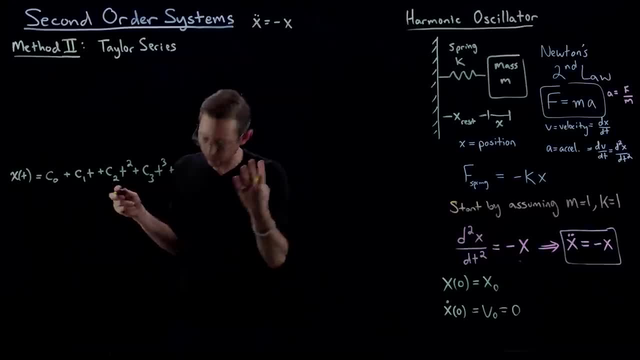 let's say i need to go up to t maximum and then let's set t plus one into t squared. so if we see that, even though, like this, is pretty easy that we're trying to justegenge one such that it's to the fourth, probably plus c4, t to the fourth, plus dot, dot, dot- this goes on forever- it's a. 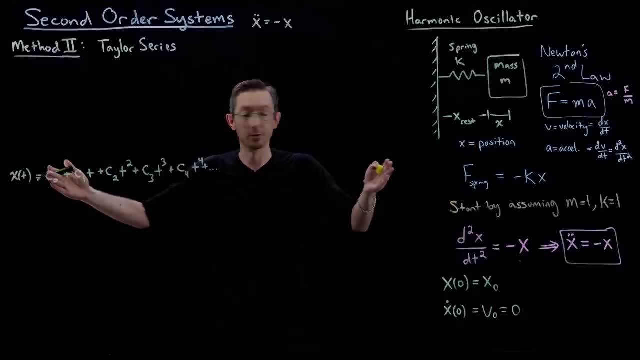 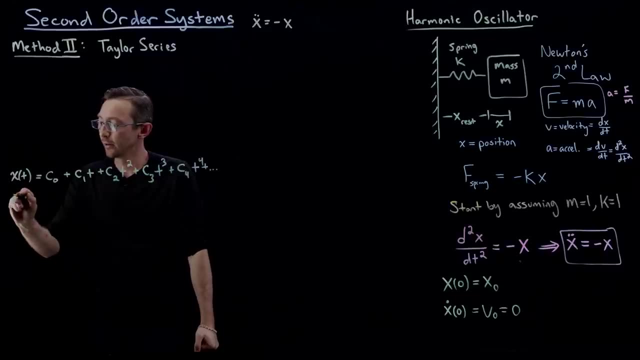 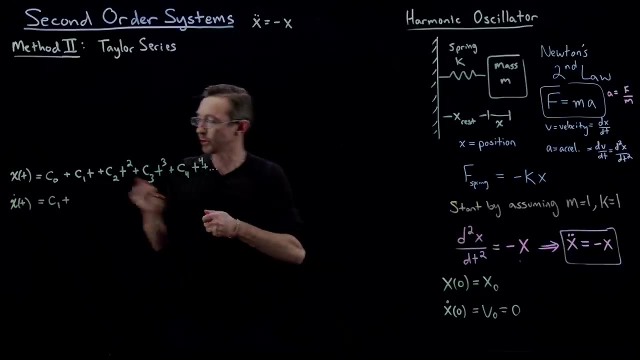 Taylor series expansion or power series expansion. so this is only you know true, if I keep all of the terms in t, and so I'm just going to compute both of its derivatives. so x dot of t is equal to now c1 plus. let's see, I can make this: orange plus 2 c, 2 t plus 3 c, 3 t squared plus 4 c, 4 t, cube plus. 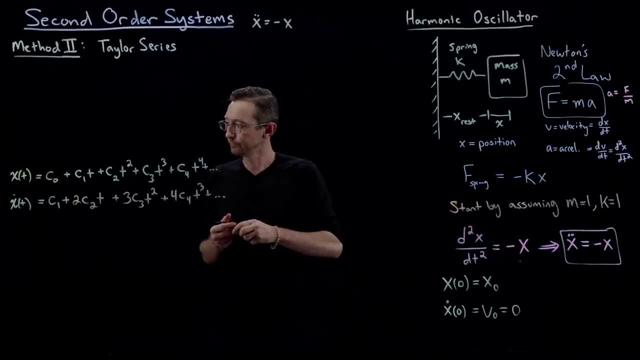 dot, dot, dot, dot dot. maybe I'll write plus 5. I'll try to keep all of the terms because I'm going to be setting them equal to each other, so I'll keep you know. plus 5 c, 5 t. plus 3 c, 3 t squared, plus 4 c, 4 t cubed. plus dot, dot, dot dot. maybe I'll write plus 5 c, 5 t. 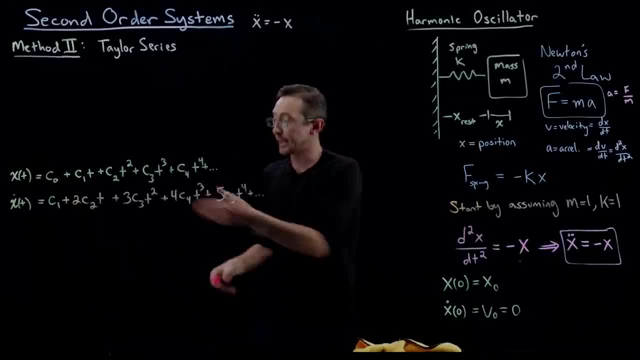 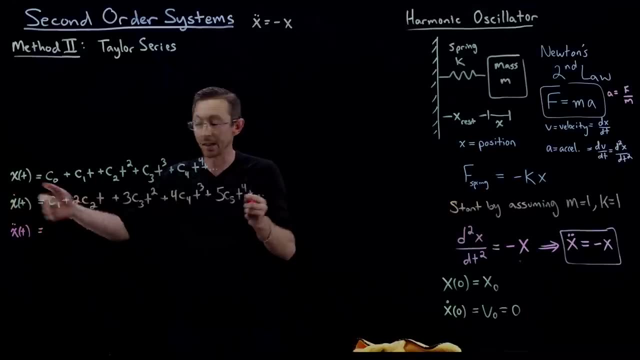 to the fourth, plus dot, dot, dot. and then the second derivative of x, dot, x double dot of t is going to now again, I'm just taking the derivative of x? dot of my velocity and this is going to equal 2 c. 2 plus 3 times 2 c, 3 t plus 4 times 3. remember the power rule: 4 times 3 c, 4 t squared plus 5. 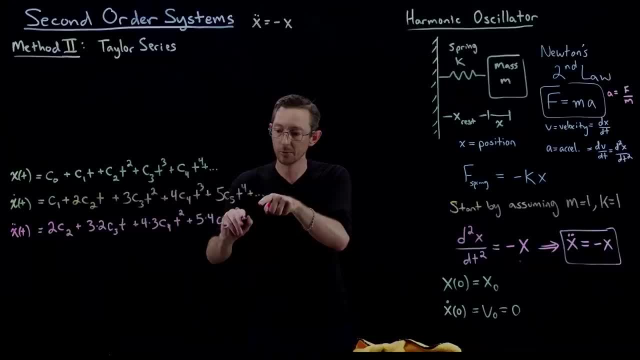 times 4 c, 5 t cubed, plus dot, dot, dot, dot dot. and if I had a third-order equation with an X triple dot, I'd have to compute X triple dot here and I would get you know more hairy terms. nothing, nothing super complicated. and now I'm literally just like we've always done: I'm going to set X double dot. 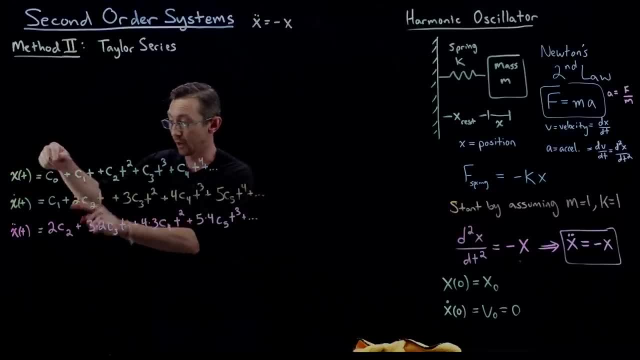 equal to minus X, and we're going to make sure that the constants at each power of T equal each other, because this has to be true for all time, which means it has to be that the the constants equal each other. the coefficients of the t to the one power equal each other. the coefficients of the 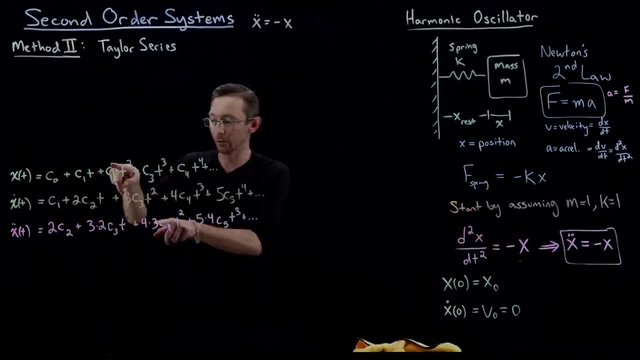 t squared terms. they have to be equal and opposite. actually they have to equal the opposite of each other, and so on and so forth. so that's going to give me a recursion relationship so that i can write down what is c2 in terms of c naught, what is c3 in terms of c1, and so on and so forth. 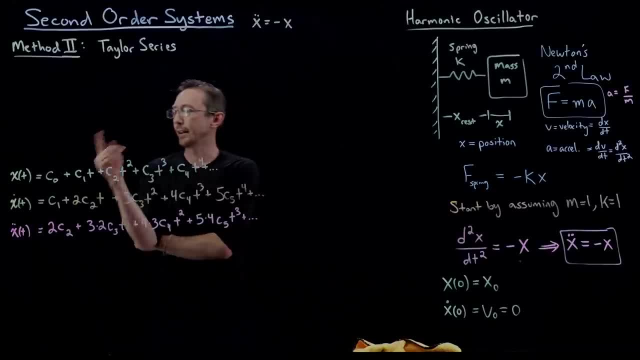 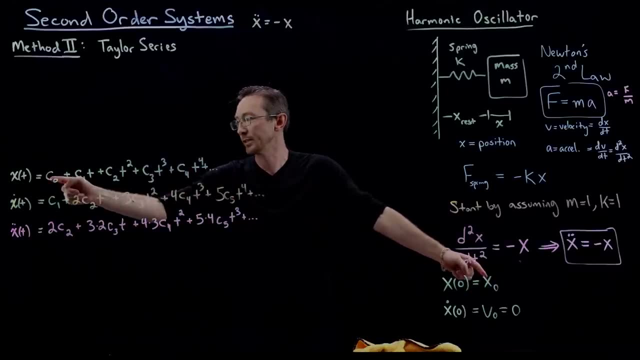 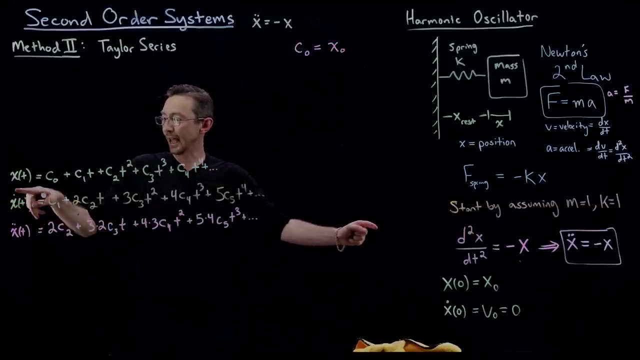 and i think i'm going to use the fact again, because x at time zero is x naught and if i plug in t zero, all of this goes to zero, except for c naught. so i probably have the relationship that um c naught equals x naught. and similarly, if i take my first derivative, x dot at time zero. 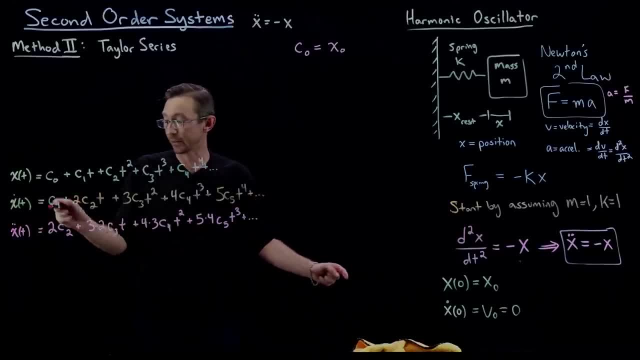 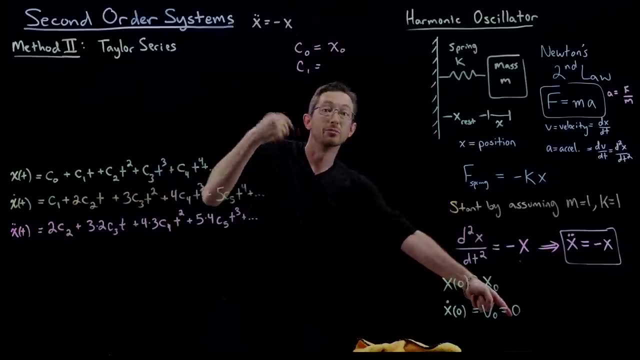 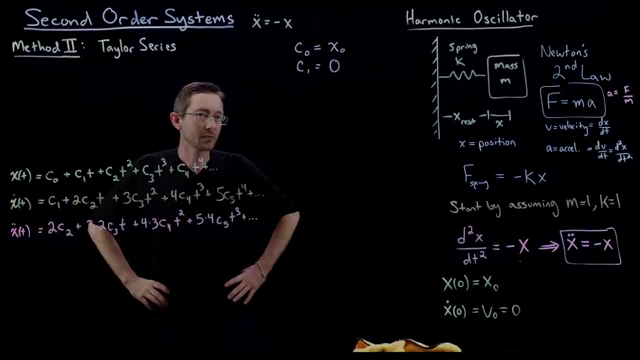 all of these terms in orange go to zero, and i'm only left with c1, and so c1 is equal to my initial velocity, which we set equal to zero. okay, so let's say this is equal to zero. good, um, you know what? let's say i had an initial velocity. this will actually be more interesting. 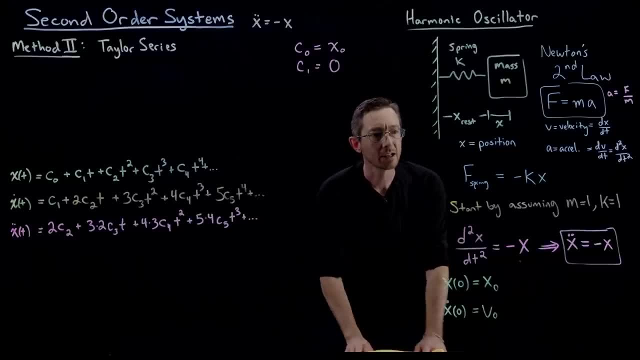 this way. um, i hope i don't butcher my notes, but let's say i actually do start with an initial velocity, so i don't just pull this mass and let it go with no velocity. i pull this mass back and i kind of push it a little. 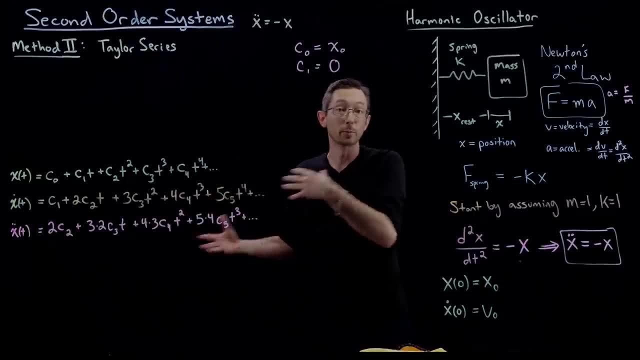 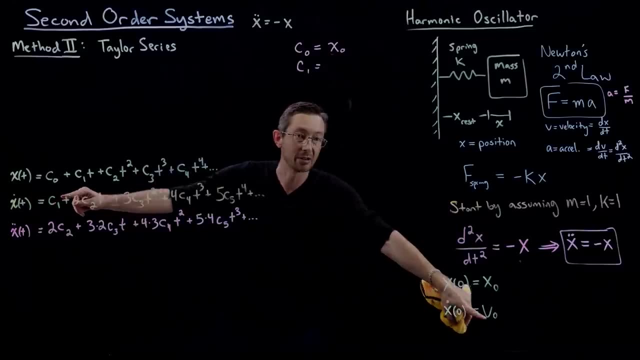 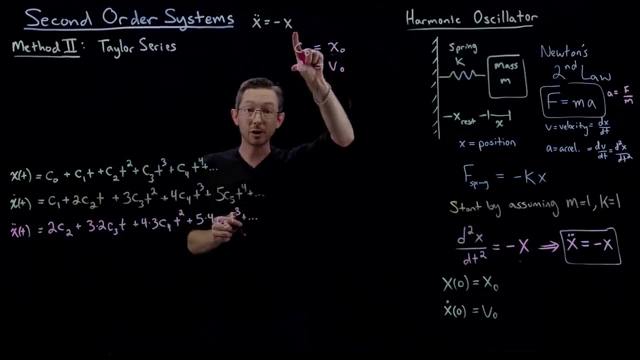 and i'm only left with c1, and so c1 is equal to my initial velocity. i give it some velocity, i give it some little initial velocity. so now it has an initial position and an initial velocity. so in that case, again, x dot at zero. c1 has to be my initial velocity. c1 has to equal v naught, and that's enough information now to 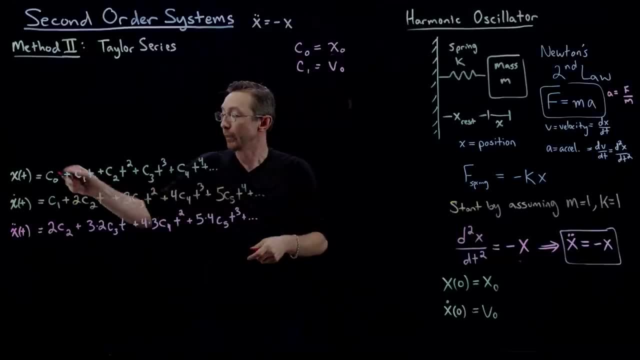 uniquely determine c2 and c3 and c4 and c5 by equating all of these uh coefficients in a recursion relation. so let's just do it. so again, remember we're writing: uh x double dot equals minus x. so that means um, i have two, i have two. c2 equals minus c naught equals minus c naught. 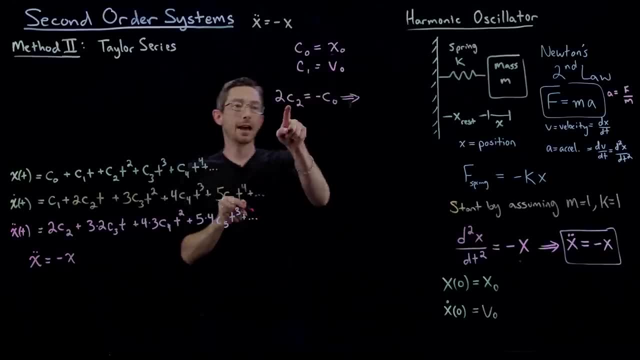 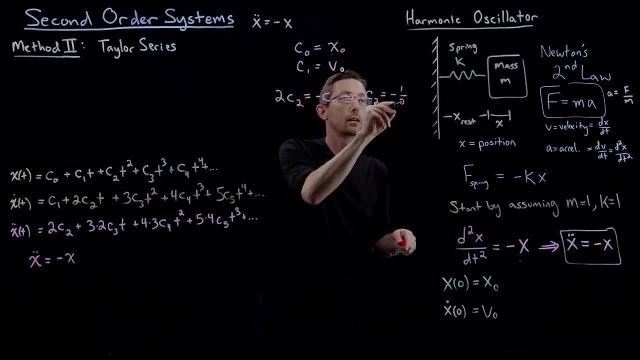 which implies that c2 equals minus one half x naught. that's pretty easy: 2 c2 equals minus x naught. so c2 equals minus one half x naught. similarly, i get my c3. this term has to equal minus this term, so i get. 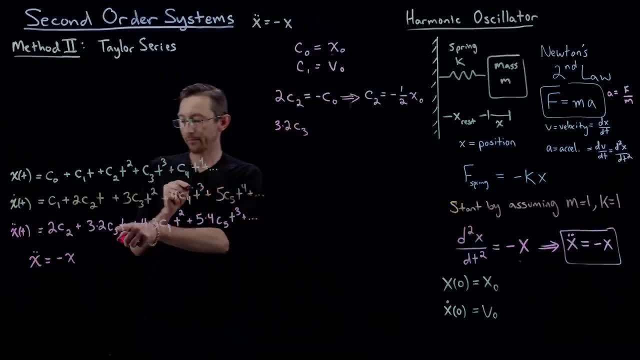 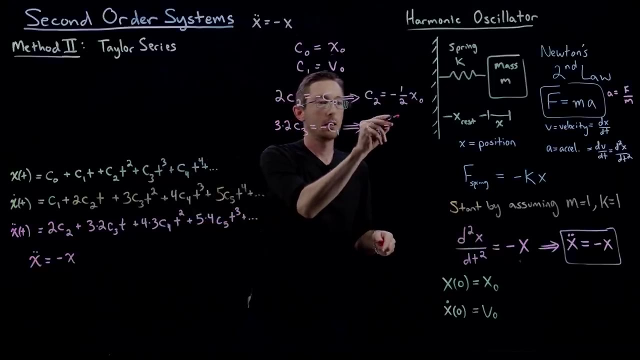 three times two. c3 equals minus c1, and again c1 is v naught, and so this equals c3 equals minus one over three times two, which i'm going to write as three factorial times v naught, and two factorial is equal to two. okay, so i've already computed my c3 and my c2. 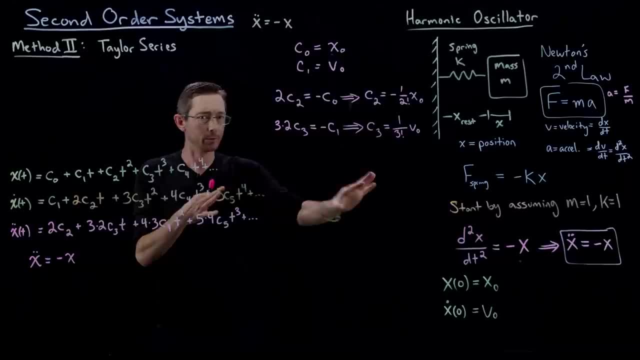 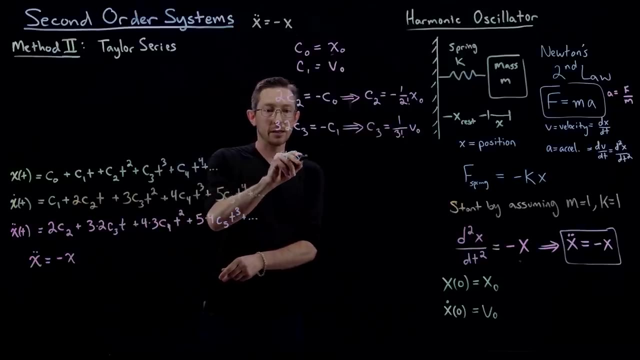 coefficient. so let's see what c4 and c5 are, and i think at that point we'll be able to stop and we'll be able to write down the solution. uh, maybe i'll switch colors here, uh, just to keep it a little neater. so my c4 coefficient is on my t squared here. so i have, uh, four times three c4. 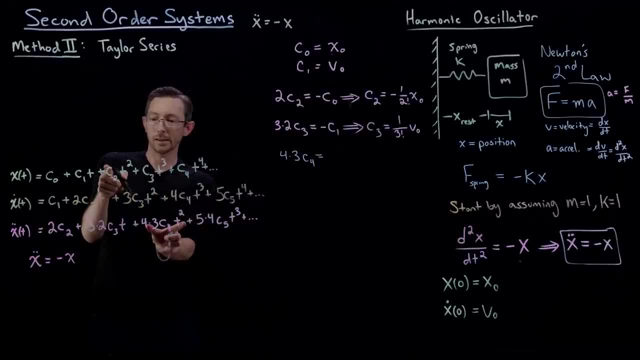 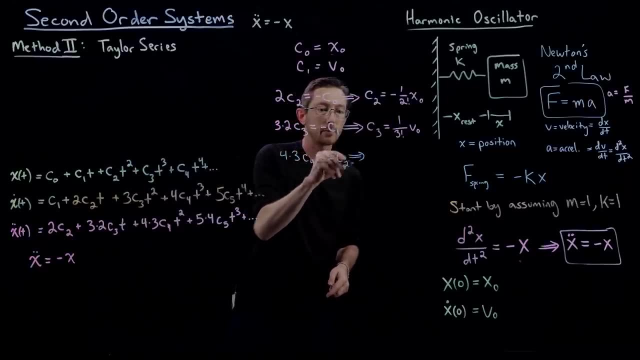 equals minus c2. that equals minus c2, because it's this equation: equals minus c2, which implies that c4 equals minus c2 divided by two, which implies: minha equatим ell gesagt, c4 equals Какие challenges um c2.. I Thumbs up if you enjoyed this video. if you'd like to support us like a little bit of financially, Please don't forget to leave us a like on the social media center. but, uh, be sure to subscribe if you want to see all of our songs, if you want to watch our videos. I just know I love you so much. thanks for sharing the content and i'll talk to y'all. I'll see y'all. bye, bye, bye. 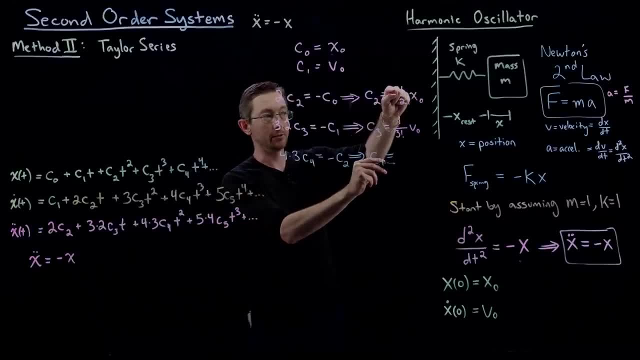 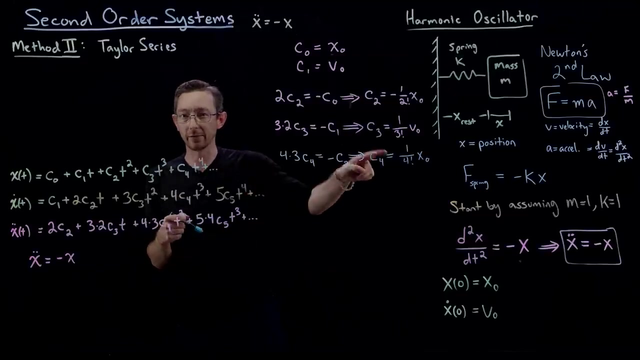 by four, divided by three and minus c two is one over two factorial times x naught. and so minus c two divided by four divided by three is one over two times three times four, which is a four factorial. okay. so, um, if that was a little fast, just pause and convince yourself that that's. 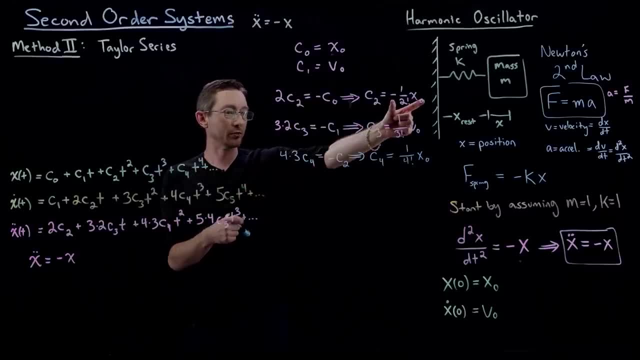 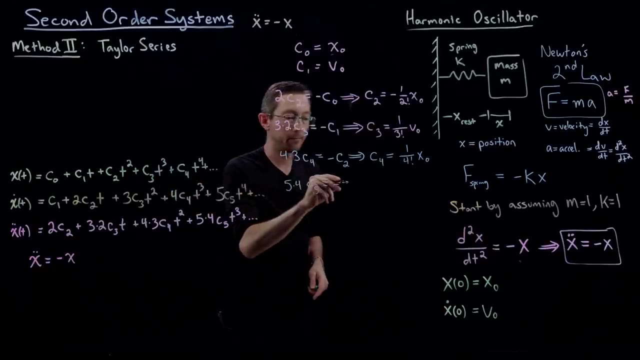 true, um, i literally take this expression for c two. i minus it and i divide by three and i divide by four and that gives me c four equals one over four. factorial x naught similarly for the c5 term. here i have five times four. c five equals minus c three. again, that's the t cube terms have to be. 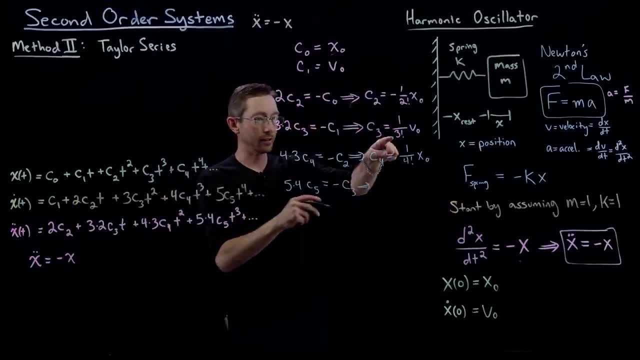 equal, and again that means i'm going to get something that looks like minus. so c5 is minus c3 divided by four, divided by five, so that's minus one over five factorial times, v, naught. and you can go, you know, on, and on, and on, and on forever, okay. so it's pretty clear what the 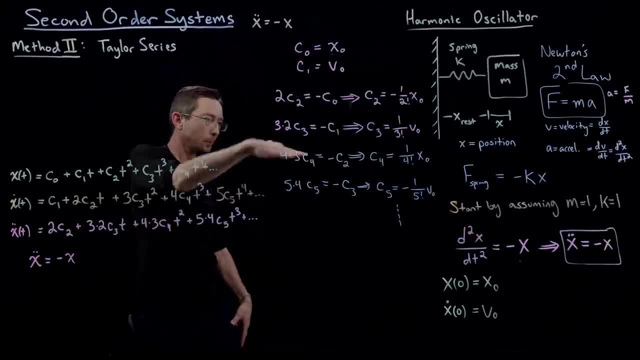 pattern here is: all of the even terms are multiplied by x knots, all of the odd terms are multiplied by v knots. and again, if you are pretty familiar with exponential functions and sines and cosines in their power series, you'll recognize pretty quickly that these are starting. 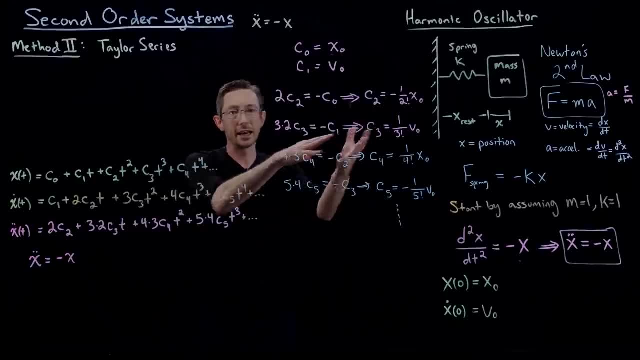 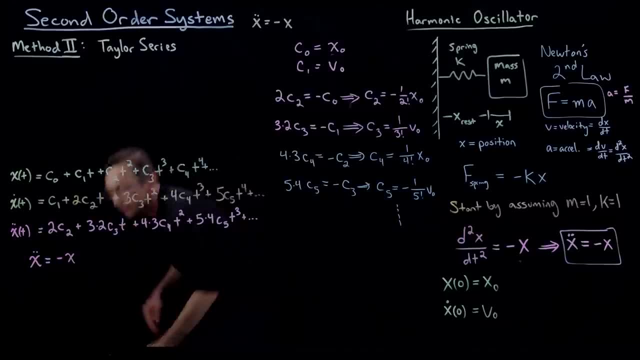 yeah, i'll do this in two steps, just because i don't want to um, i don't want to confuse anyone. so what i'm going to do, the first thing i'm going to do is i'm literally just going to write x of t, um and plug in all of those coefficients here, and then i'm going to group all of my x naughts. 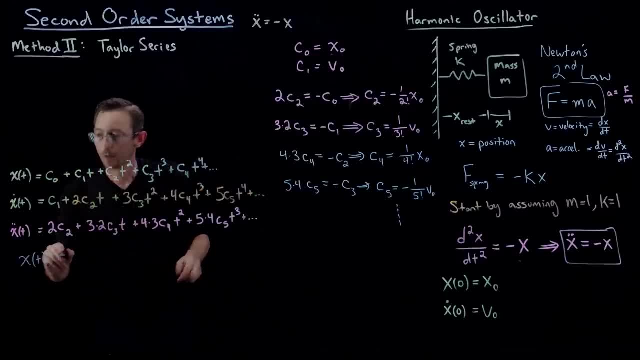 and my v naughts. so x of t equals x naught plus v naught t. c2 is minus 1 over 2 factorial x naught times t. squared, c3 is- i feel like i'm missing a minus sign. yeah, this is supposed to be minus, right? this is a c3 equals minus c1, so there's a minus there. 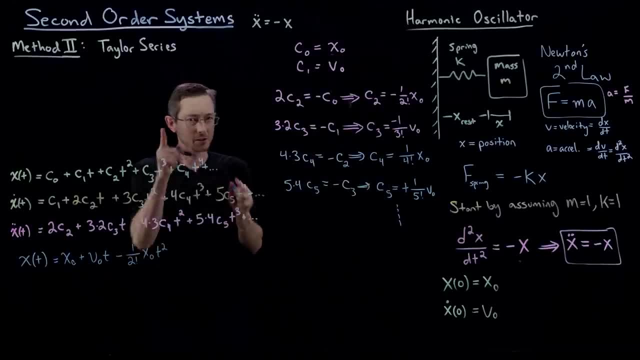 and c5 is minus c3, so this is a plus sign. okay, thank you. i'm sure many of you caught that um, so sorry, my um. i already have my c2 now. my c3 term is minus 1 over 3. factorial v naught t cubed. 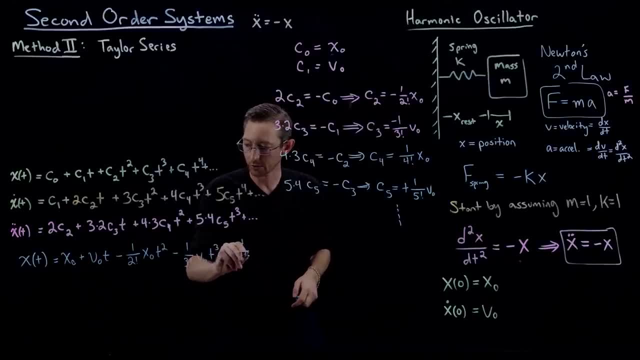 and i'm going to have, uh, plus 1 over 4 factorial x- naught again t to the fourth. plus 1 over 5 factorial v- naught t to the fifth. minus dot, dot, dot dot. okay, this is literally. i'm just taking this expression here and i'm plugging in what we got from our recursion relationship. 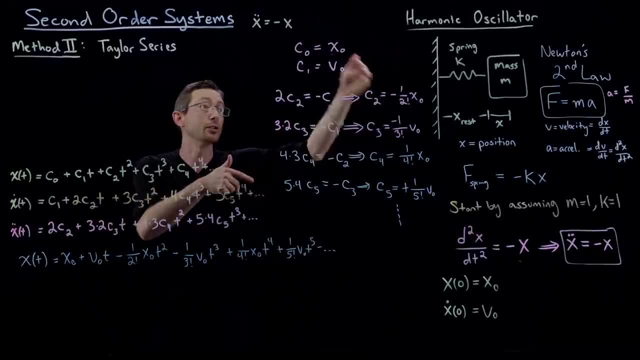 from our recurrence relationship for all of these constants. okay, in terms of x- naught and v- naught, and now i can take all of the terms that are only functions of x- naught, and i can take all of my terms that are only functions of v- naught and i can write those down. 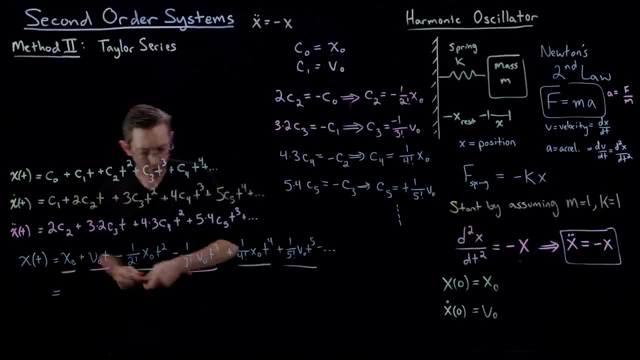 and i can say that x of t equals- maybe i'll write this in yellow- i get x naught times one, minus t, squared over two factorial plus t to the fourth over four factorial, you know, minus, i'm sure it's going to be t to the six over six, factorial plus dot, dot dot. 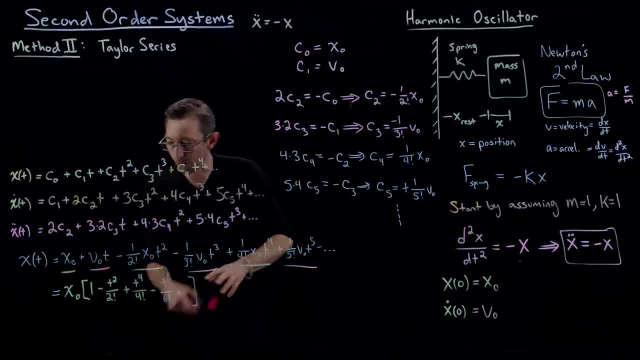 okay, that's all of my terms, that are x knots, and then i'm also going to get plus v naught times, all of these, these odd powers in t. okay, so i'm going to get v naught times t minus 1 over 3 factorial t. cubed plus 1 over 5 factorial t to the fifth. dot, dot, dot, dot dot. 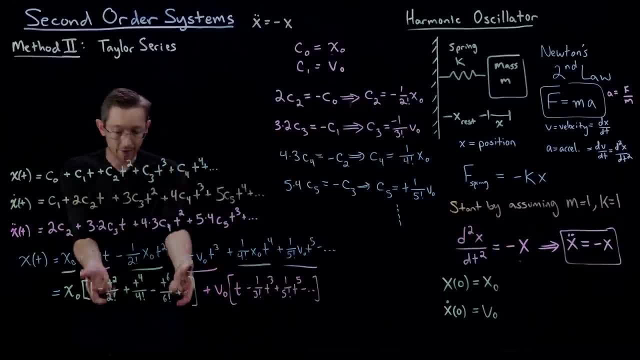 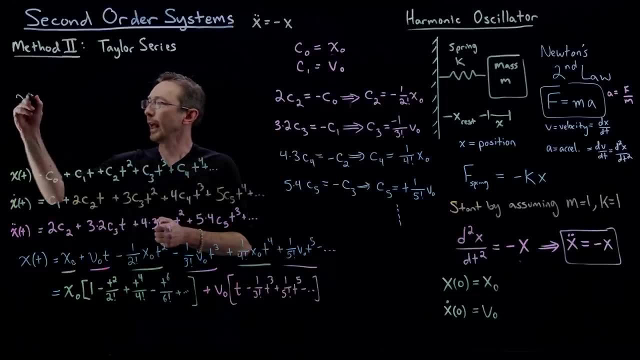 forever and ever and ever. and lo and behold, this is the taylor series for cosine and this is the taylor series for sine. and so what we find is that x of t equals the yellow for my cosine. this is cosine of t times x, naught times my initial position. 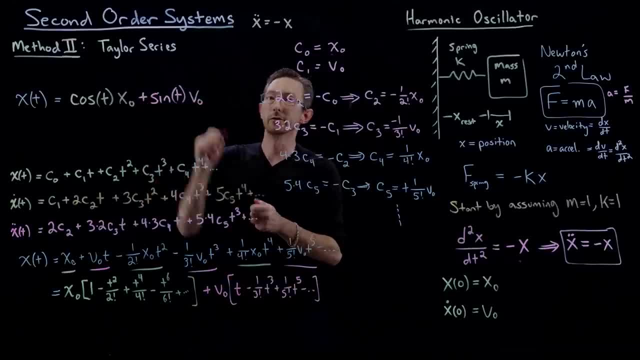 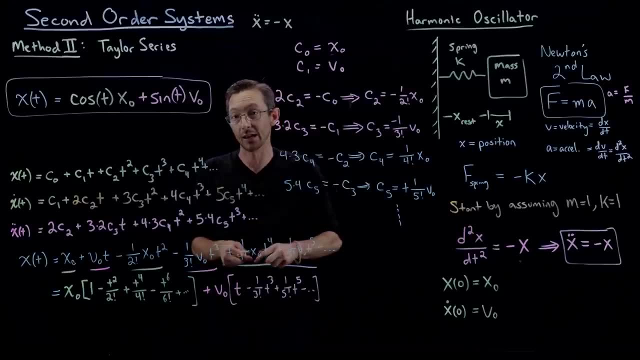 plus sine of t times my initial velocity, and that is the solution to this differential equation. now for a generic initial position and initial velocity. so remember when i guessed i had to use the simple case where there was zero initial velocity, or else i might have messed up my guess. when you do the taylor series, you can actually have your initial position and an. 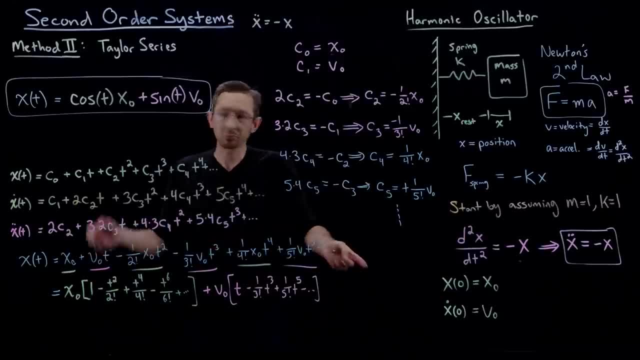 initial velocity and it just kind of pops out that you get cosine times the initial position plus sine times the initial velocity. so these are kind of out of phase. so if i start with, you know, some initial position and an initial velocity, this is my generic solution. good, okay, um, that was. 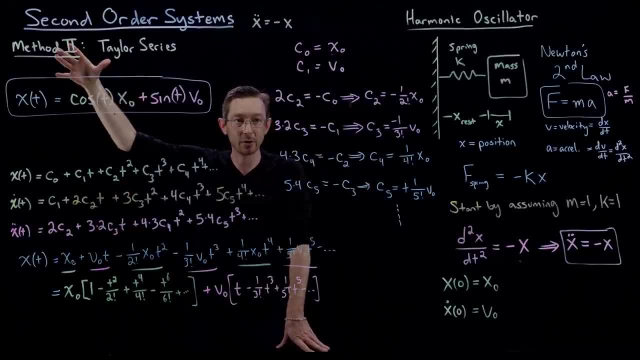 method two, and this is again not recommended to use this every day when you're solving differential equations, but really important to know that almost every solution of every differential equation you'll ever see, you could solve it using the kind of first principles, Taylor series, power series, expansions, good, okay. method. 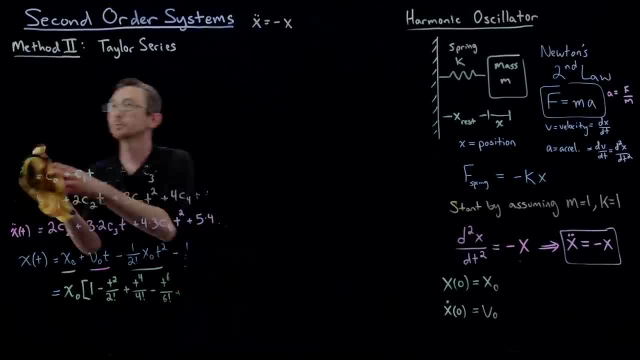 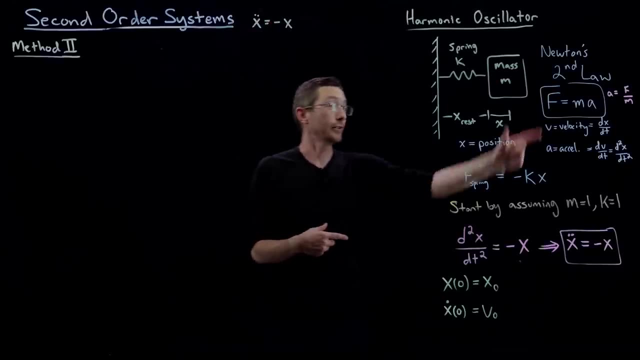 three. I'm gonna erase this and we're gonna solve method three. okay, we are solving this second-order differential equation which we derived from Newton's second law. F equals ma for the position of this mass on a spring. so X is the position, X double dot is its acceleration and the force of the spring. 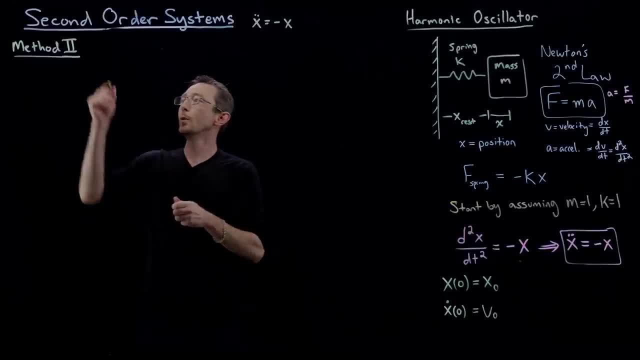 is minus X. so this is the differential equation. we've already solved this two ways. now we're gonna solve it a third way. so the first time we just guessed cosine solutions because you know that seemed reasonable, given that it's oscillating, it's a, you know, springy mass. the second solution was Taylor series. we 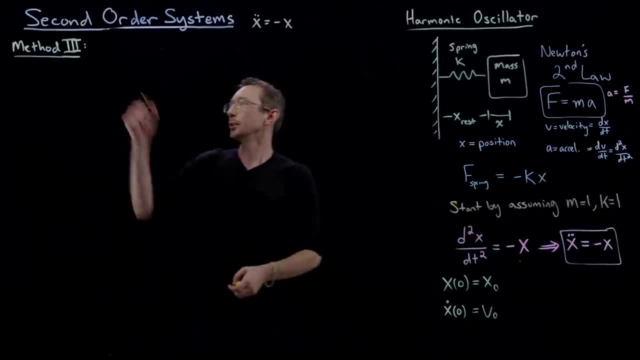 actually wrote out a Taylor series expansion for X of T. the third method: we're gonna guess again. we're gonna guess again. but instead of guessing that our solution X of T is some cosine solution, we're gonna guess again. but instead of guessing that our solution X of T is some cosine solution, we're. 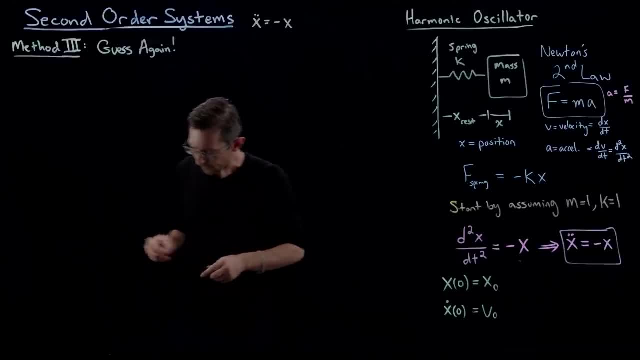 going to guess something a little different. so remember what function, when we take its derivatives, are, up until a constant looks like itself. so in first order, systems X dot equals lambda X. we saw that the exponential function was the very natural solution, because if I take the derivative of e to the lambda, 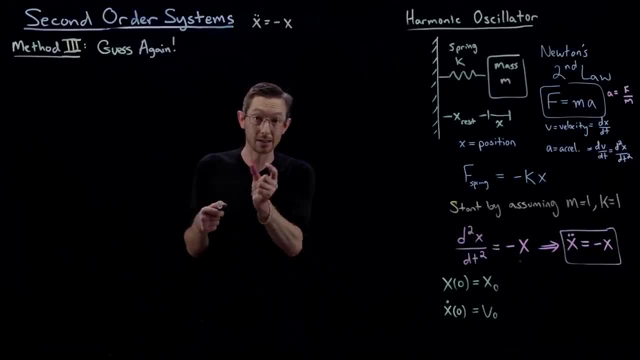 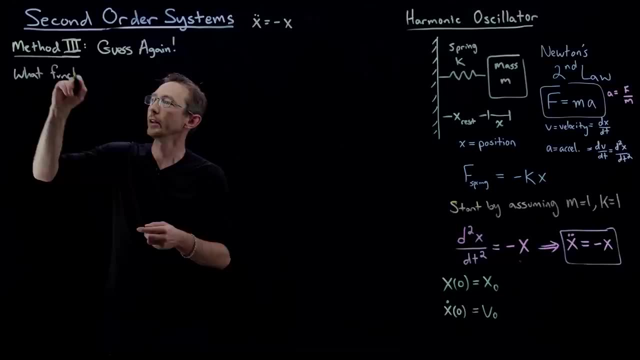 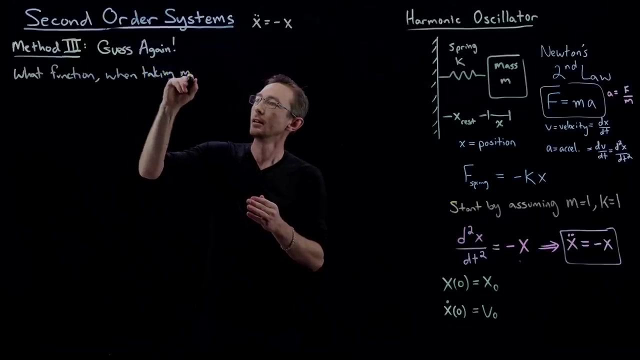 you know, T, I get something that up to a constant is also e to the lambda T. just remember, you know I'll write this out, remember, you know I'll write this out. what function: what function when taking? what function? what function when taking? multiple derivatives when taking. 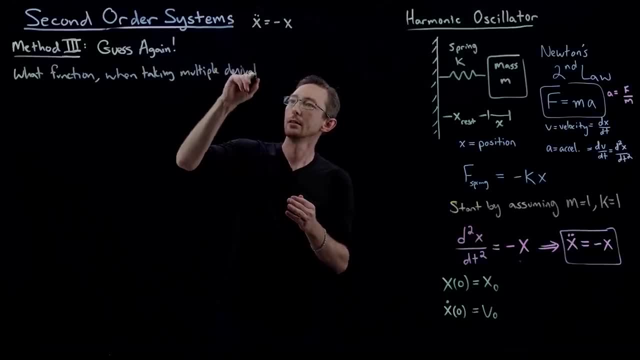 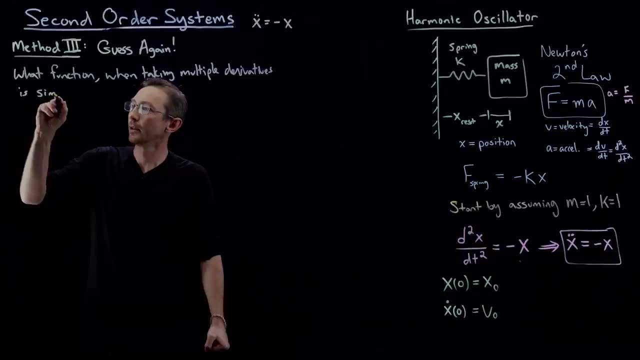 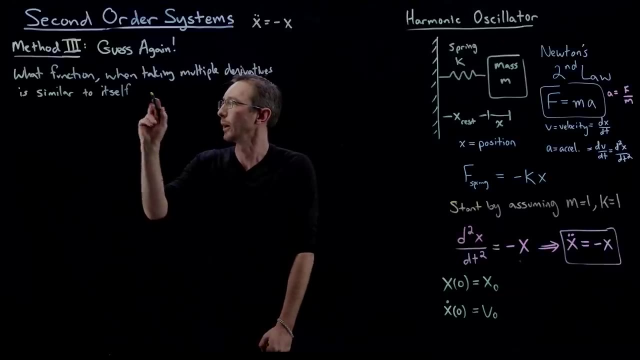 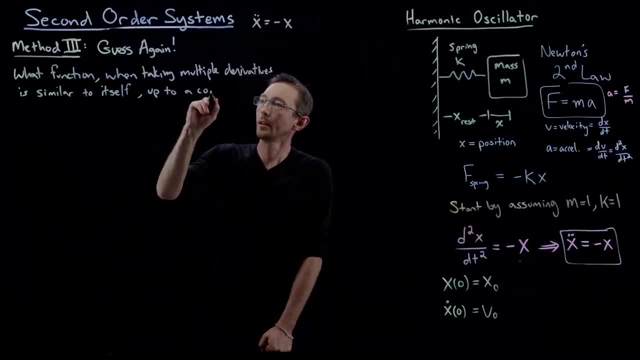 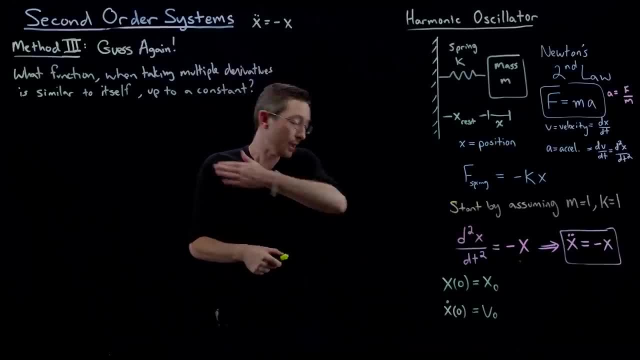 up to a constant. we know that the answer is the up to a constant. we know that the answer is the exponential function. I can take exponential function. I can take exponential function. I can take the derivative of e to the T as many times the derivative of e to the T as many times. 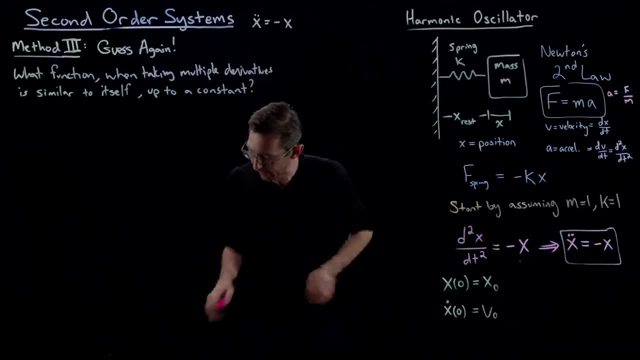 the derivative of e to the T as many times as I want, and I get exactly e to the as I want, and I get exactly e to the as I want, and I get exactly e to the T back. so you know, X of T equals e to the. 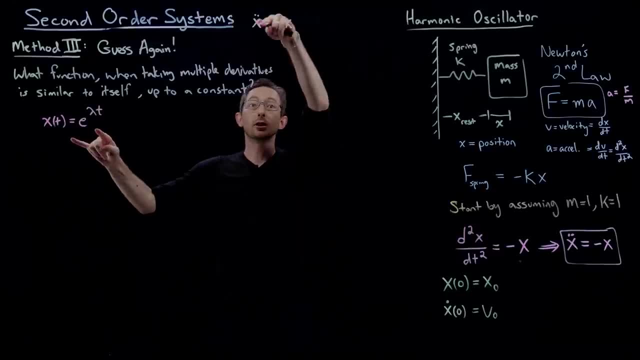 T back. so you know X of T equals e to the T back. so you know X of T equals e to the. lambda T is a pretty good guess for lambda T is a pretty good guess for lambda T is a pretty good guess for the solution of differential equations. 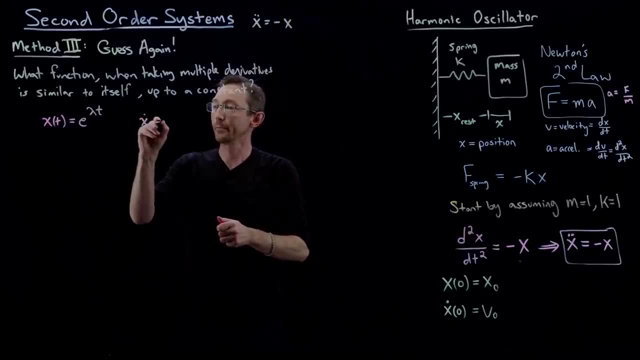 the solution of differential equations. the solution of differential equations, because if I take the second derivative, because if I take the second derivative, because if I take the second derivative, let's write this down- X dot is going to. let's write this down: X dot is going to. 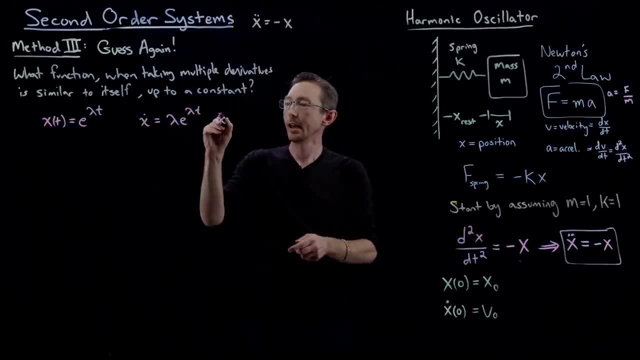 let's write this down: X dot is going to be lambda. e to the lambda T and X be lambda. e to the lambda T and X be lambda. e to the lambda T and X. double dot is going to be lambda squared. double dot is going to be lambda, squared. 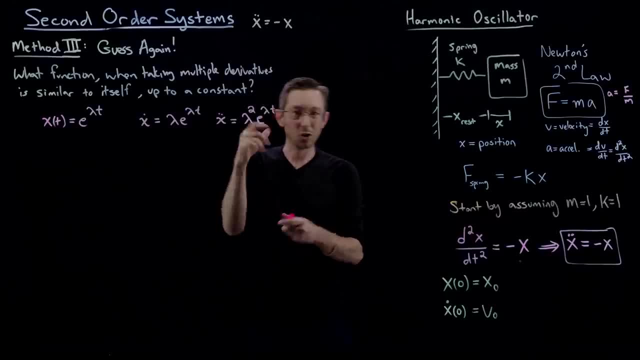 double dot is going to be lambda, squared e to the lambda T. so I always get e to the lambda T, so I always get e to the lambda T. so I always get something that looks just like itself, something that looks just like itself, something that looks just like itself, and so I can kind of again equate these. 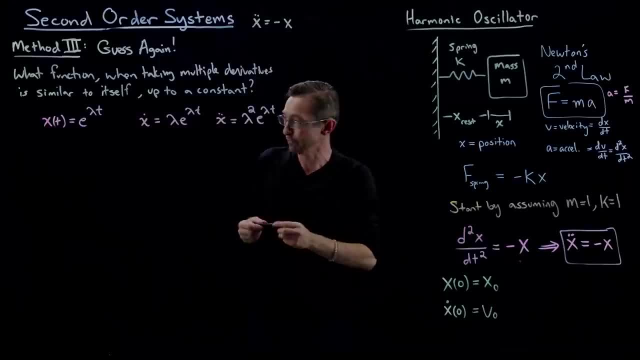 and so I can kind of again equate these. and so I can kind of again equate these two equal and opposite to each other. I two equal and opposite to each other, I two equal and opposite to each other. I can plug these two into this equation. 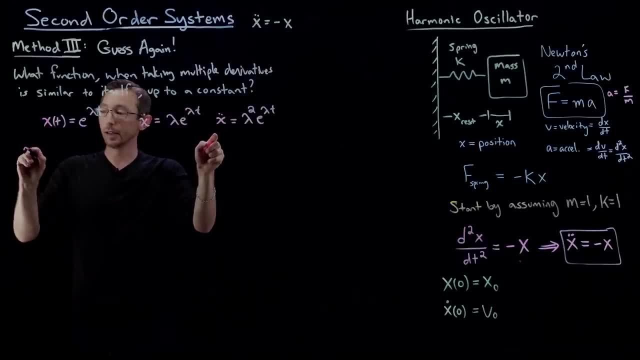 can plug these two into this equation. can plug these two into this equation. and I get that lambda squared e to the and I get that lambda squared e to the and I get that lambda squared e to the lambda T. better equal minus e to the lambda T better equal minus e to the. 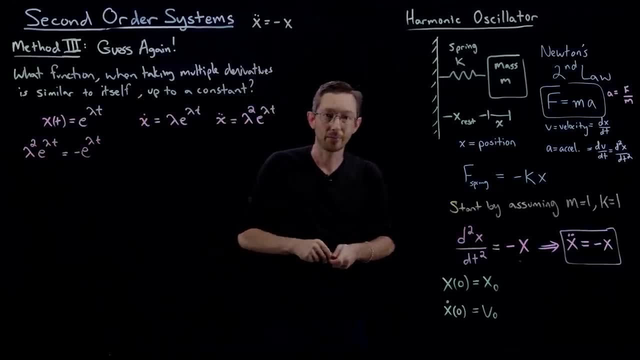 lambda T better equal minus e to the lambda T. that's just X. double dot equals lambda T. that's just X, double dot equals lambda T. that's just X. double dot equals minus X, and of course this has to be minus X and of course this has to be. 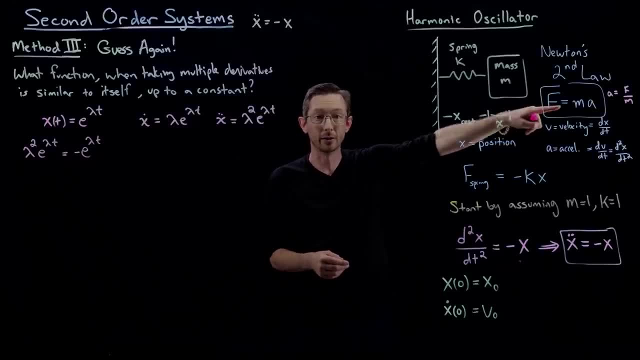 minus X and of course this has to be true for all times. because Newton second, true for all times. because Newton second, true for all times, because Newton second law doesn't ever take any breaks. it law doesn't ever take any breaks. it law doesn't ever take any breaks. it never goes to sleep, it never has sick. 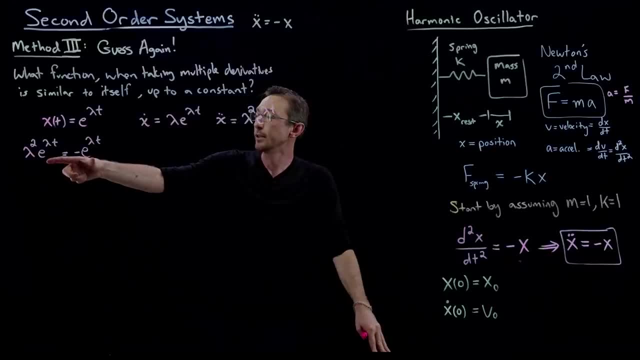 never goes to sleep. it never has sick. never goes to sleep. it never has sick days. it's true for all time that we're days. it's true for all time that we're days, it's true for all time that we're aware of, and so this is true for all of. 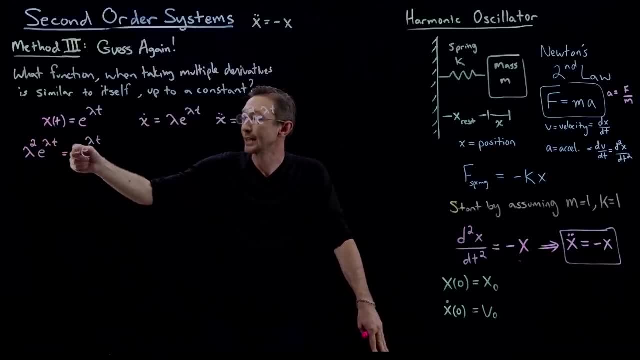 aware of, and so this is true for all of aware of, and so this is true for all of these. e to the lambda T's, which means these. e to the lambda T's, which means these. e to the lambda T's, which means that lambda squared has to equal minus. 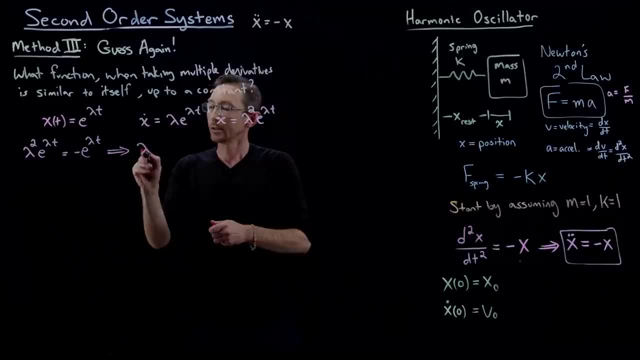 that lambda squared has to equal minus, that lambda squared has to equal minus one. that's the only way that this can be one. that's the only way that this can be one. that's the only way that this can be true. so lambda squared equals minus one. 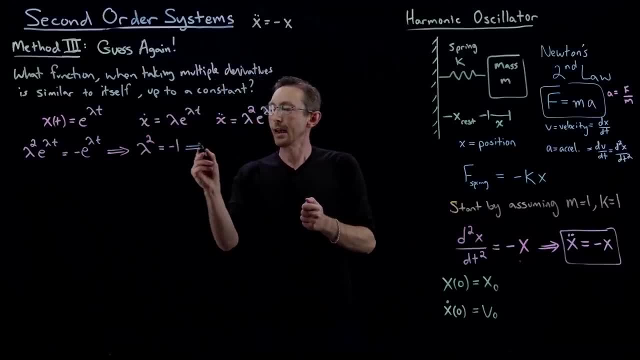 true, so lambda squared equals minus one. true, so lambda squared equals minus one, which means I'll switch colors here. that which means I'll switch colors here. that which means I'll switch colors here, that means that lambda equals the square root. means that lambda equals the square root. 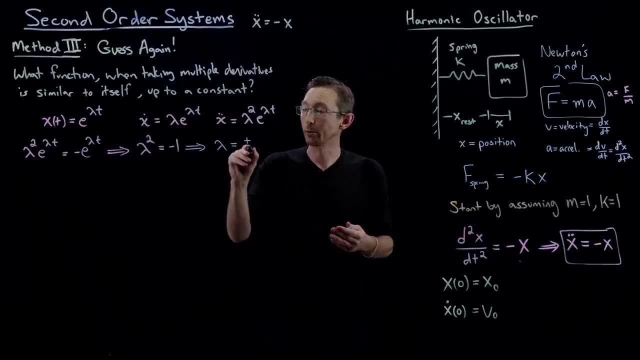 means that lambda equals the square root of minus one which is plus or minus I, so of minus one which is plus or minus I, so of minus one which is plus or minus I. so lambda could equal plus I or minus I, and lambda could equal plus I or minus I, and. 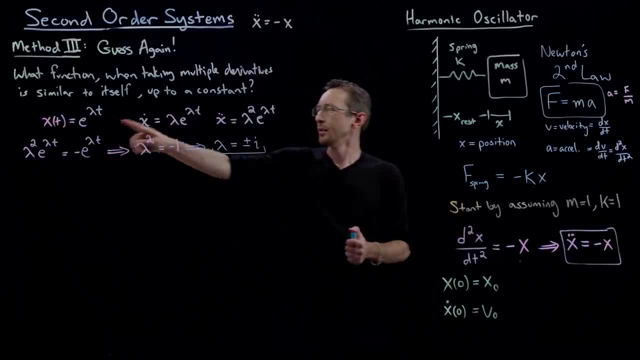 lambda could equal plus I or minus I, and this is really interesting now, what we- this is really interesting now. what we- this is really interesting now what we have- is that our solution X of T is have, is that our solution X of T is have, is that our solution X of T is going to be written in terms of e to. 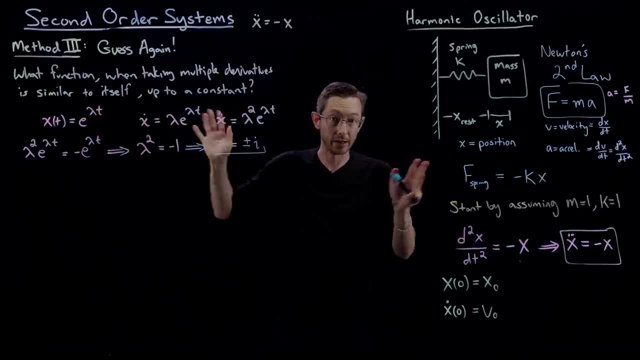 going to be written in terms of e to going to be written in terms of e to the plus I T's and e to the minus I T's, the plus I T's, and e to the minus I T's, the plus I T's, and e to the minus I T's. very, very interesting, because this is a. 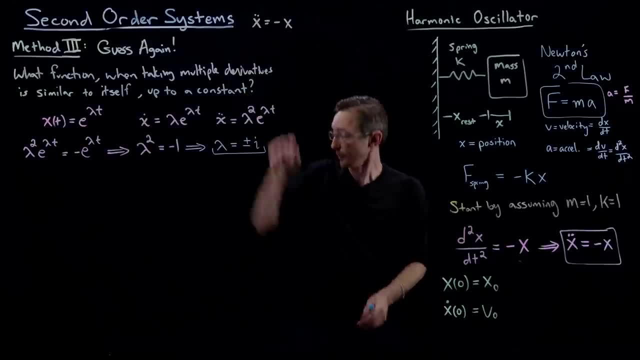 very, very interesting, because this is a very, very interesting, because this is a linear differential equation. meaning that linear differential equation, meaning that linear differential equation, meaning that the derivative- okay, that was not a drill, apparently. okay, that was not a drill, apparently. okay, that was not a drill, apparently, those were fire alarms. okay, because this. 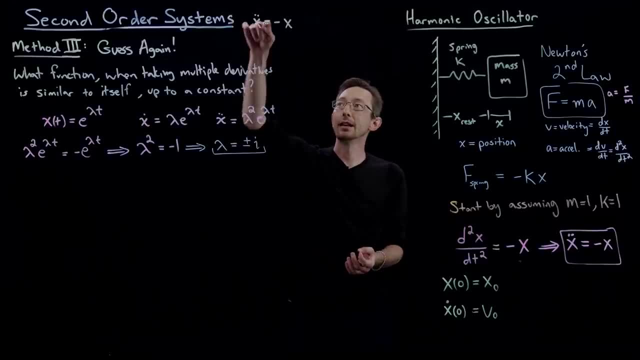 those were fire alarms. okay, because this, those were fire alarms. okay, because this differential equation is linear meaning. differential equation is linear meaning. differential equation is linear meaning that the meaning that the meaning that the derivatives are linearly proportional to the state X, derivatives are linearly proportional to the state X. 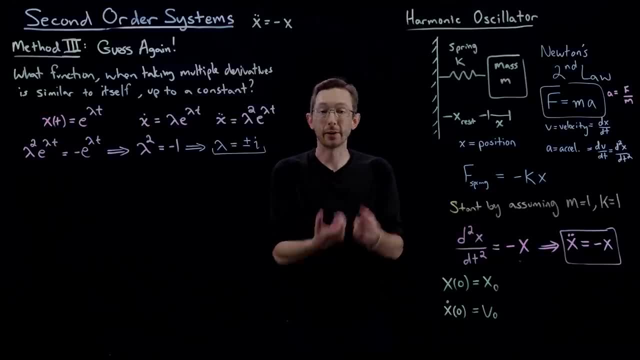 derivatives are linearly proportional to the state X. that means the linear, that means the linear, that means the linear superposition holds. so if I have two superposition holds, so if I have two superposition holds, so if I have two solutions to the system, then if I add 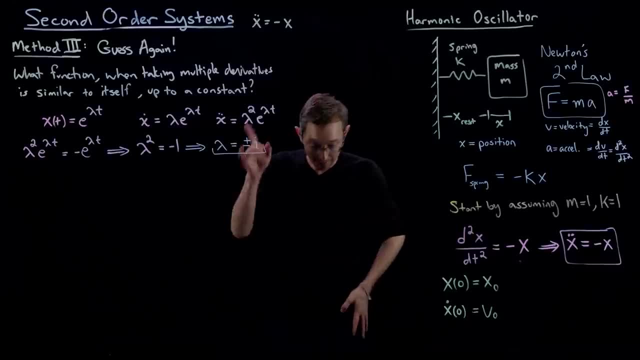 solutions to the system, then if I add solutions to the system, then if I add those solutions up, that's also a those solutions up, that's also a those solutions up, that's also a solution to the system. and so what? that solution to the system, and so what that? 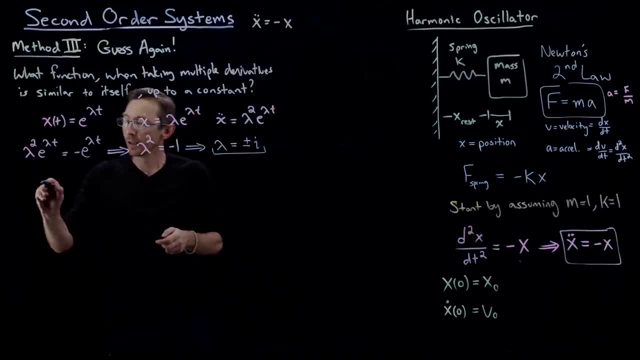 solution to the system, and so what that means is that the candidate for X of T means, is that the candidate for X of T means, is that the candidate for X of T is now X of T. it could be e to the plus- is now X of T, it could be e to the plus. 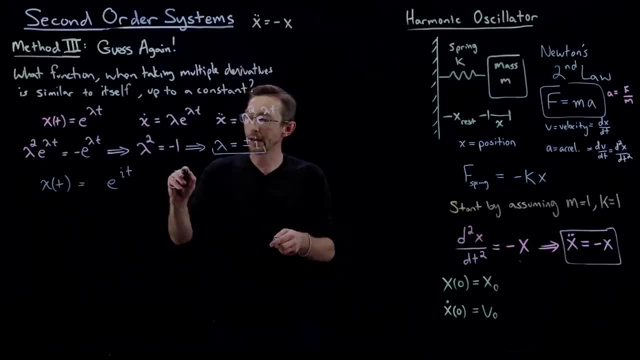 is now X of T. it could be e to the plus I T, or it could also be e to the minus I I T, or it could also be e to the minus I I T, or it could also be e to the minus I T. if I took either of those solutions, 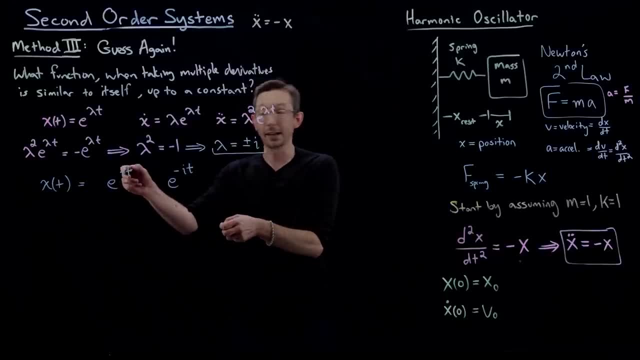 T if I took either of those solutions, T if I took either of those solutions and I took the second derivative and I took the second derivative and I took the second derivative literally. you know the second derivative literally. you know the second derivative literally. you know the second derivative of e to the I, T is minus e to the IT, or. 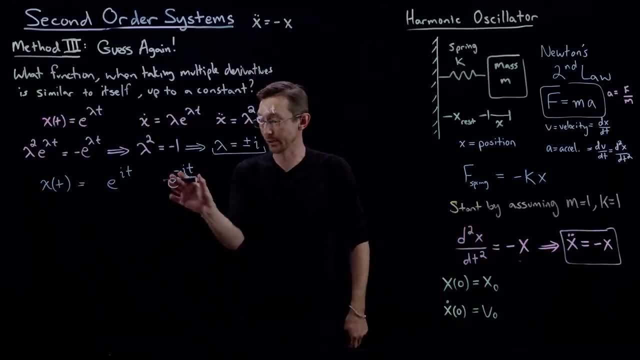 of e to the I T is minus e to the IT, or of e to the I T is minus e to the IT, or I square e to the IT is a solution of my I square e to the IT is a solution of my I square e to the IT is a solution of my differential equation. and so is this so. 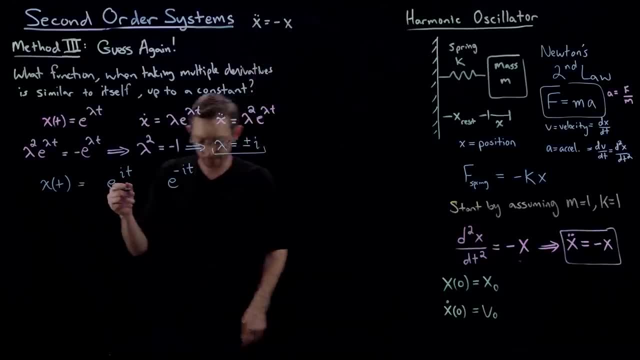 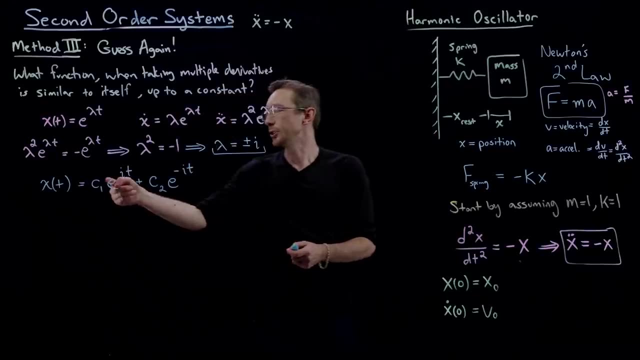 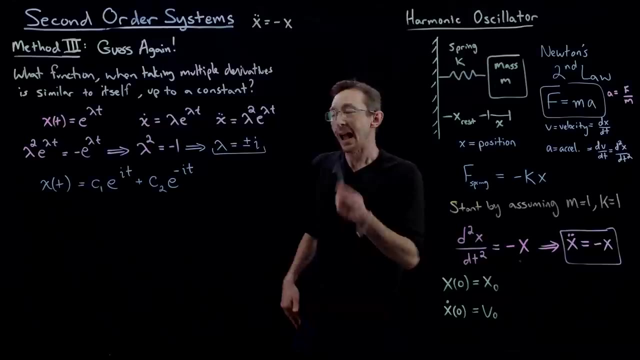 differential equation. and so is this so differential equation, and so is this so in the coefficients c1 and c2, based on: in the coefficients c1 and c2, based on in the coefficients c1 and c2, based on our initial conditions, and specifically our initial conditions, and specifically: 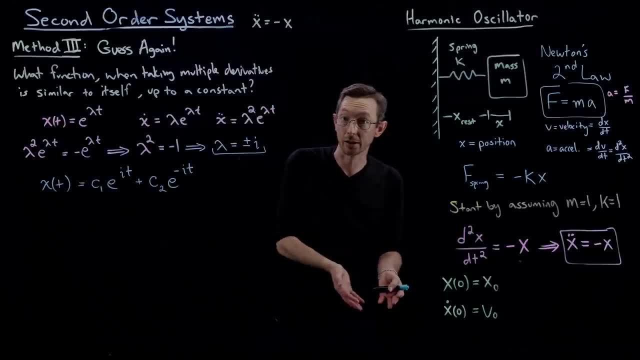 our initial conditions and specifically, you know e to the I T is gonna have a. you know e to the I T is gonna have a. you know e to the I T is gonna have a real part and an imaginary part, and so real part and an imaginary part, and so. 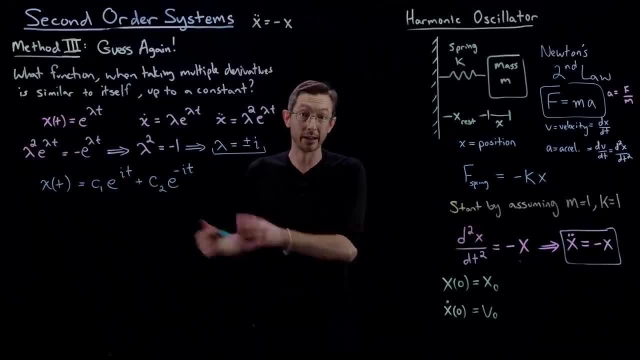 real part and an imaginary part, and so I'm gonna also choose c1 and c2, so that I'm gonna also choose c1 and c2, so that I'm gonna also choose c1 and c2, so that it basically is only a real valued. 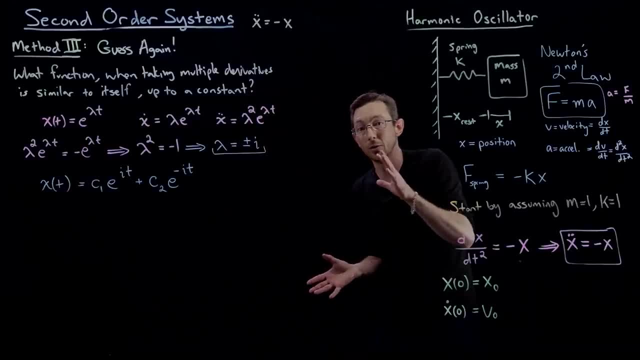 it basically is only a real valued. it basically is only a real valued function because of course you know if I function. because of course you know if I function, because of course you know, if I pull this mass and let it go, I can't get. pull this mass and let it go, I can't get. 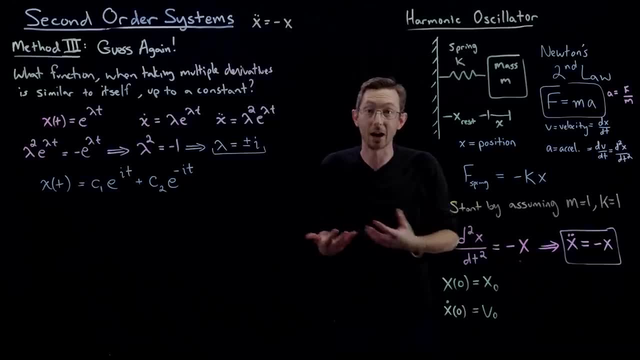 pull this mass and let it go. I can't get an imaginary position or an imaginary, an imaginary position or an imaginary, an imaginary position or an imaginary velocity. I can't get a complex valued velocity. I can't get a complex valued velocity. I can't get a complex valued position or velocity, and so these: 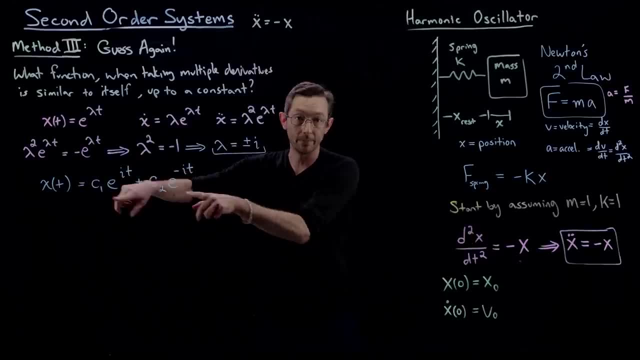 position or velocity, and so these position or velocity and so these coefficients have to perfectly add up. so coefficients have to perfectly add up. so coefficients have to perfectly add up so that only the real part of these, that only the real part of these, that only the real part of these functions remains. okay, that's kind of. 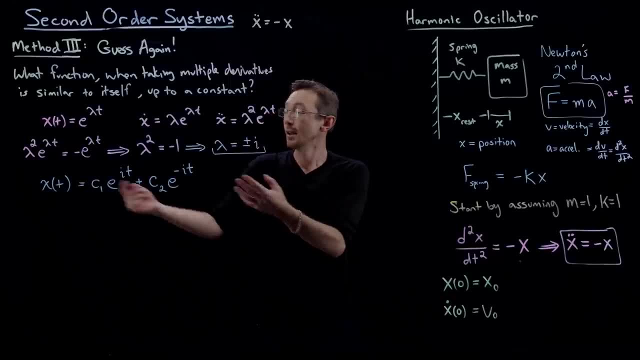 functions remains okay. that's kind of functions remains okay. that's kind of interesting that you know. I now have interesting that you know. I now have interesting that you know I now have these complex lambdas, but of course my, these complex lambdas, but of course my. 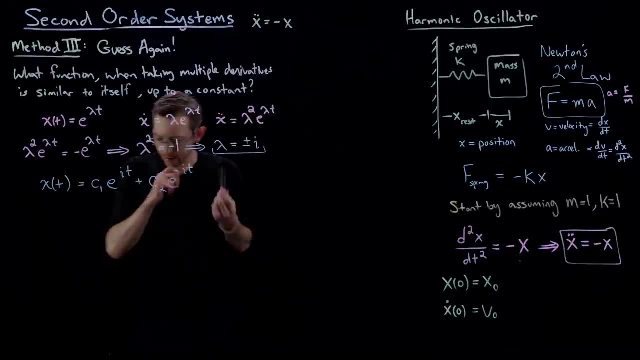 these complex lambdas, but of course, my position and velocity are still going to position and velocity are still going to position and velocity are still going to be real. so let's do this. and so now I be real. so let's do this. and so now I. 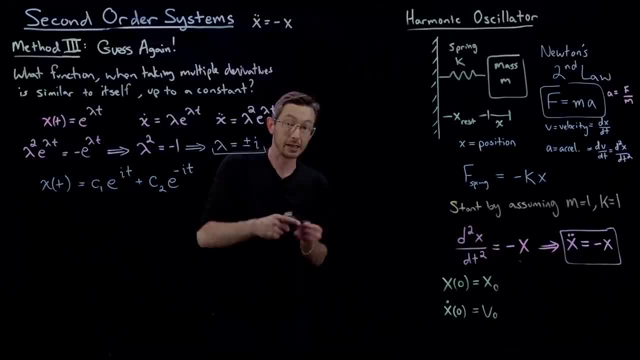 be real. so let's do this. and so now I know that e to the IT is cosine T plus I know that e to the IT is cosine T plus I know that e to the IT is cosine T plus I sine of T, and so I can write this as you. 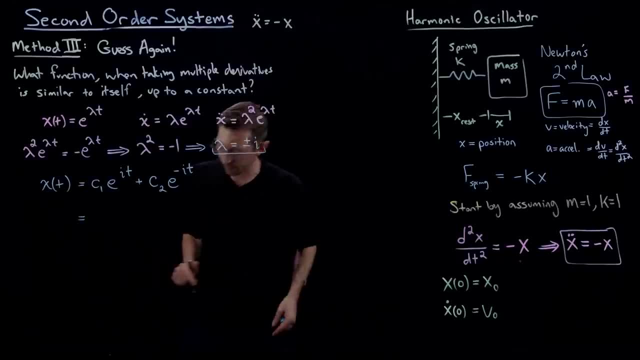 sine of T, and so I can write this as you sine of T, and so I can write this: as you know, I can basically write down the real know. I can basically write down the real know. I can basically write down the real part and the imaginary part. I'm gonna 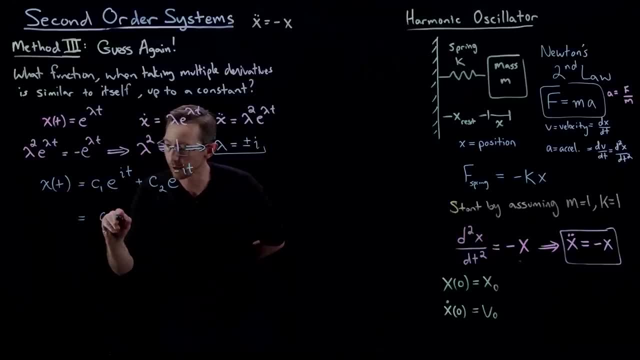 part and the imaginary part. I'm gonna part and the imaginary part. I'm gonna get something like C 1 plus C 2 times. get something like C 1 plus C 2 times. get something like C 1 plus C 2 times cosine of T plus I times C 1 minus C 2. 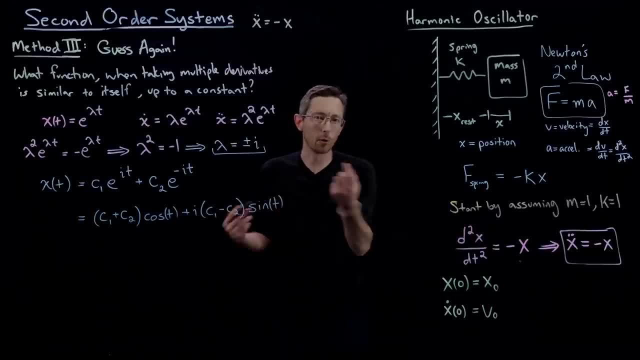 cosine of T plus I times C 1 minus C 2. cosine of T plus I times C 1 minus C 2 times sine of T. and this is just using times sine of T, and this is just using times sine of T, and this is just using Euler's formula, literally. that you know. 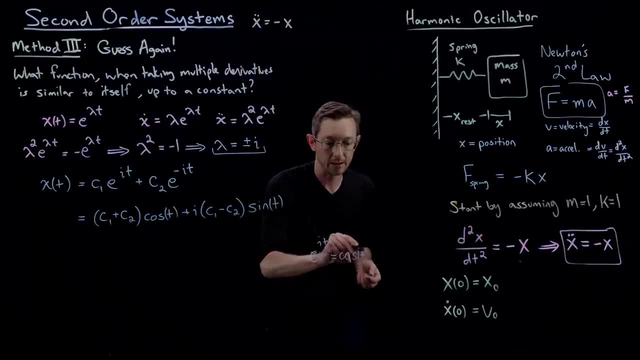 Euler's formula, literally that you know. Euler's formula, literally that you know: e to the IT equals cosine of T plus I. e to the IT equals cosine of T plus I. e to the IT equals cosine of T plus I sine of T. so similarly, e to the minus. 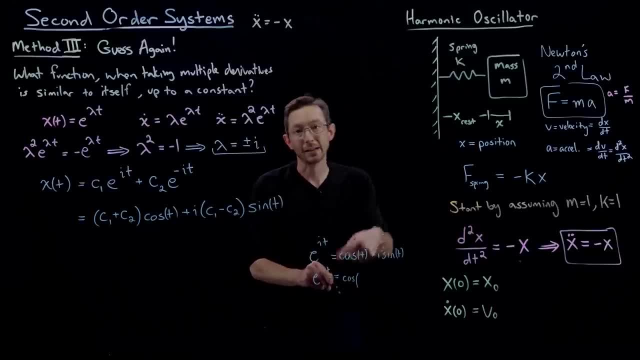 sine of T, so similarly e to the minus. sine of T, so similarly e to the minus. IT equals cosine of minus T, but cosines. IT equals cosine of minus T, but cosines. IT equals cosine of minus T, but cosines, even so, that's also cosine of T plus I. 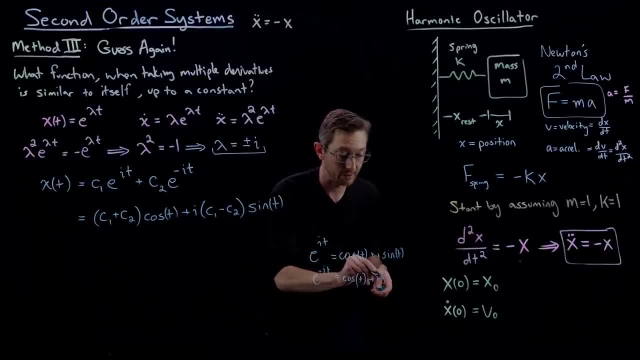 even so, that's also cosine of T plus I. even so, that's also cosine of T plus I sine of minus T. that's odd. so it's minus sine of minus T, that's odd. so it's minus sine of minus T, that's odd. so it's minus I sine of T, and you can plug these in. 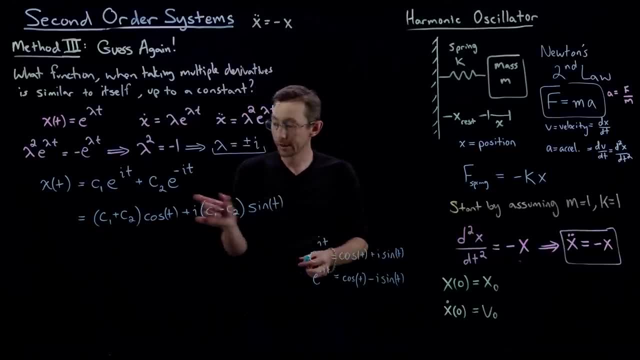 I sine of T and you can plug these in I sine of T, and you can plug these in here and get this expression. so now I here and get this expression. so now I here and get this expression. so now I can use C 1 and C 2 to essentially give. 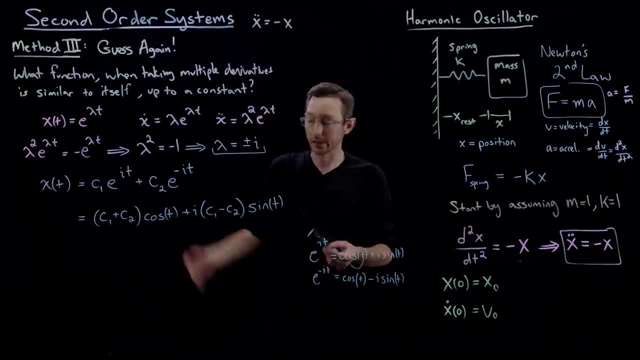 can use C 1 and C 2 to essentially give. can use C 1 and C 2 to essentially give me the initial conditions that I'm me, the initial conditions that I'm me, the initial conditions that I'm looking for. okay, and let's see, is there? 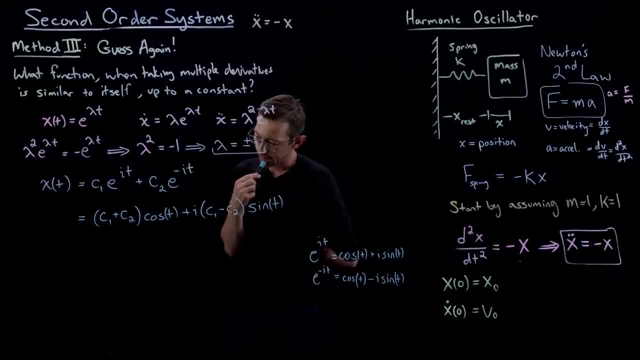 looking for, okay, and let's see: is there looking for? okay, and let's see, is there something technically, these constants, something technically, these constants, something technically? these constants could be complex, valued or real valued, could be complex valued or real valued, could be complex valued or real valued, and so I think what I'm going to find is and so I think what I'm going to find is, and so I think what I'm going to find is: yeah, okay, let's just, let's just work it. yeah, okay, let's just, let's just work it. yeah, okay, let's just, let's just work it out. I don't know what the answer is. 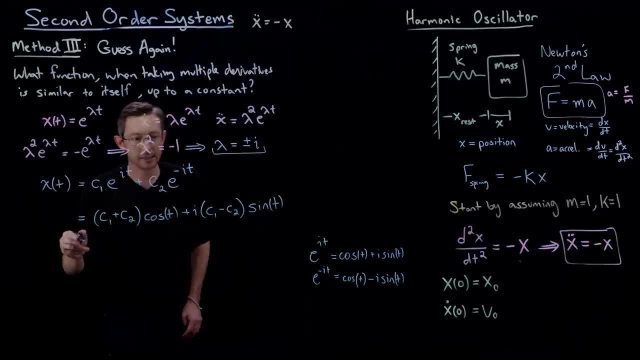 out. I don't know what the answer is out. I don't know what the answer is. we're gonna try it, so we have some. we're gonna try it, so we have some. we're gonna try it, so we have some. initial condition is that you know X at. 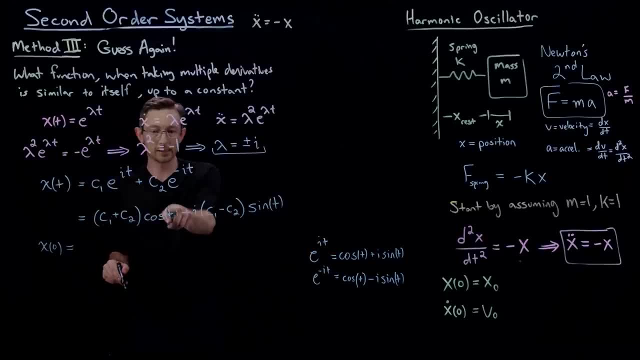 initial condition is that you know X at. initial condition is that you know X at times. 0 is going to be just you know. times 0 is going to be just you know. times 0 is going to be just you know. cosine of 0 is 1, sine of 0, 0, so that. 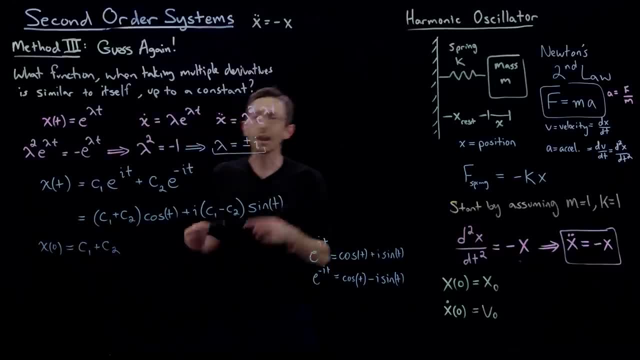 cosine of 0 is 1 sine of 0, 0, so that cosine of 0 is 1 sine of 0, 0, so that equals C 1 plus C 2, and similarly if I, equals C 1 plus C 2, and similarly if I. 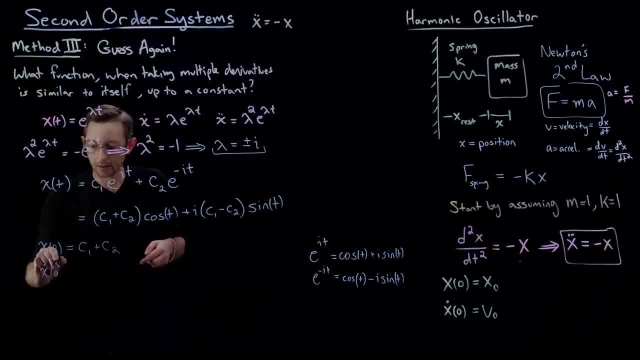 equals C 1 plus C 2. and similarly, if I take the derivative of this, you know X. take the derivative of this, you know X. take the derivative of this, you know X. dot at 0. the derivative of cosine is dot at 0. the derivative of cosine is: 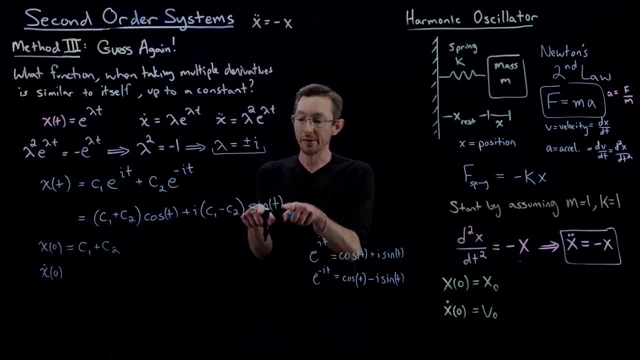 dot at 0. the derivative of cosine is minus sine and sine of 0, 0. so this term minus sine and sine of 0, 0. so this term minus sine and sine of 0, 0, so this term will be 0 and this will be cosine of T. 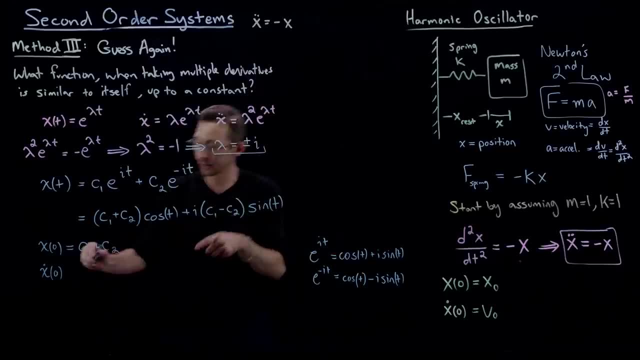 will be 0 and this will be. cosine of T will be 0 and this will be cosine of T. cosine of 0 will be 1, so X dot at 0 is. cosine of 0 will be 1, so X dot at 0 is. 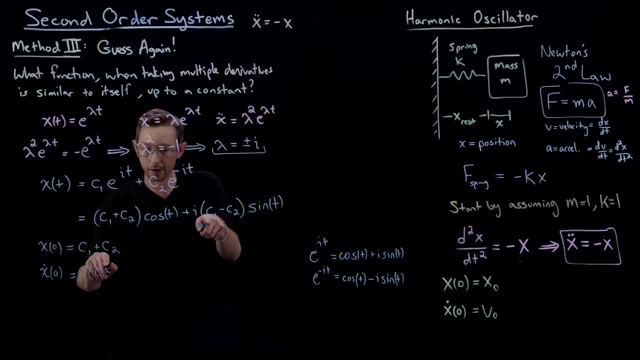 cosine of 0 will be 1, so X dot at 0 is going to equal I times C 1 minus C 2, and going to equal I times C 1 minus C 2, and going to equal I times C 1 minus C 2, and so what that means is that C 1 plus C 2. 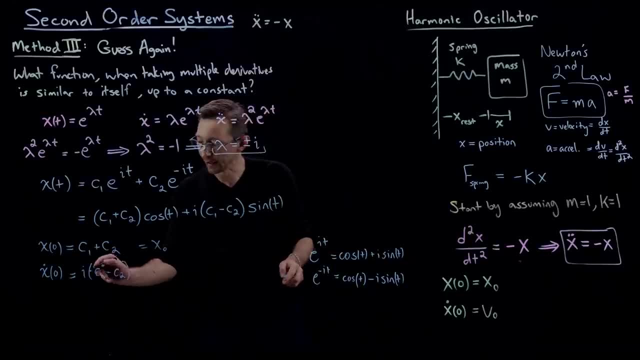 so what that means is that C 1 plus C 2. so what that means is that C 1 plus C 2 has to equal my initial position and I has to equal my initial position and I has to equal my initial position and I times C 1 minus C 2 has to equal my. 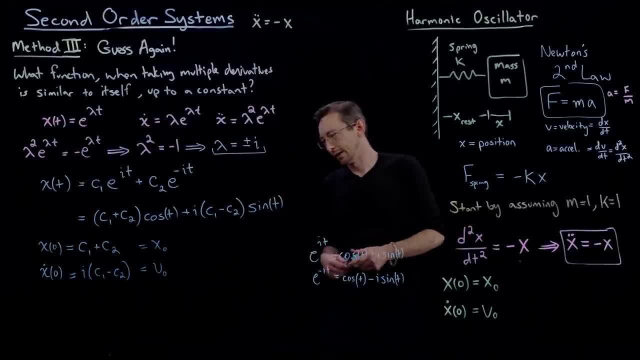 times C 1 minus C 2 has to equal my times C 1 minus C 2, has to equal my initial velocity and probably I could initial velocity and probably I could initial velocity and probably I could figure out using you know complex, figure out using you know complex. 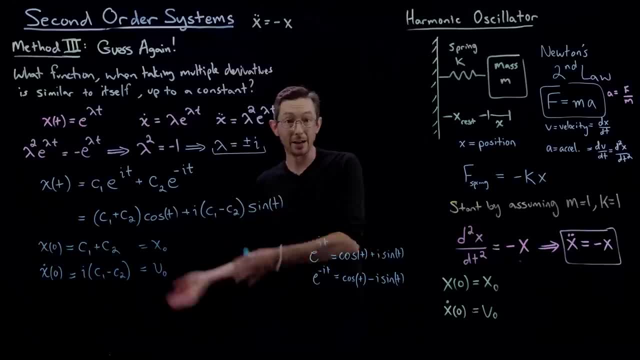 figure out, using, you know, complex analysis, that these coefficients have, a analysis that these coefficients have, a analysis that these coefficients have a real and an imaginary part, and I could real and an imaginary part, and I could real and an imaginary part, and I could, you know, figure out exactly how to make. 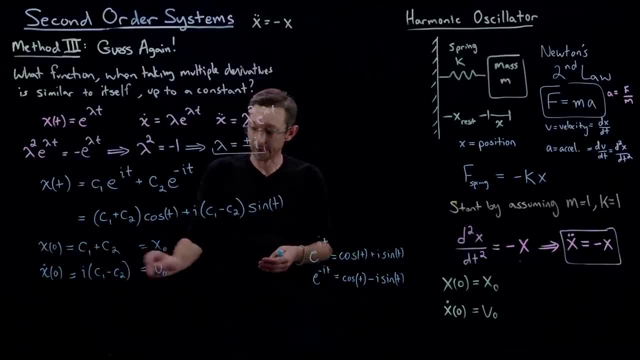 you know. figure out exactly how to make. you know, figure out exactly how to make these add up to equal a. you know real X. these add up to equal a. you know real X. these add up to equal a. you know real X not. and they're their difference times. I. 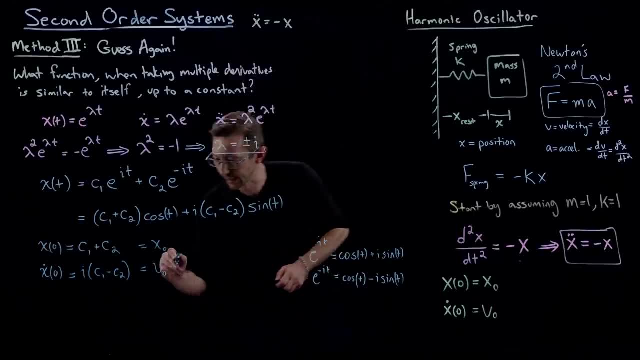 not, and they're their difference times. I not, and they're their difference times. I would equal a real V, naught. I'm just would equal a real V, naught. I'm just would equal a real V naught. I'm just gonna punt a little and say, let's, let's. gonna punt a little and say let's, let's gonna punt a little and say let's, let's imagine that V naught equals zero. so I imagine that V naught equals zero. so I imagine that V naught equals zero. so I just start this thing with an initial. 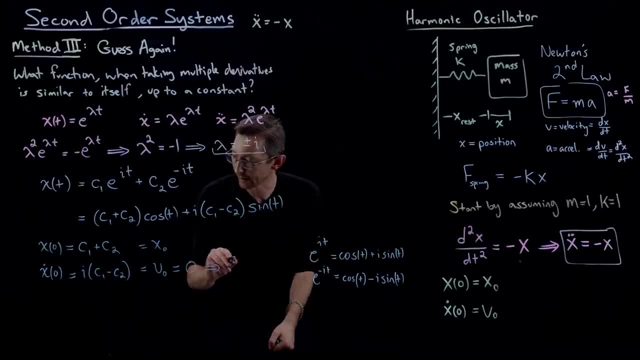 just start this thing with an initial, just start this thing with an initial position, and let it go. then that means position, and let it go, then that means position, and let it go, then that means that C 1 has to equal C 2. okay for this. 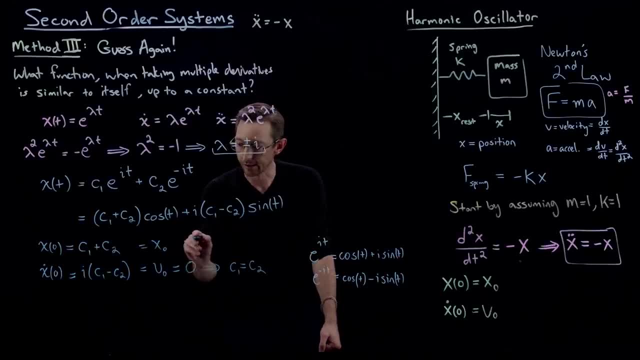 that C 1 has to equal C 2. okay for this. that C 1 has to equal C 2. okay for this to equal 0. and that means that C 1 to equal 0 and that means that C 1 to equal 0, and that means that C 1 equals C 2. so C 1 equals C, 2 equals X. 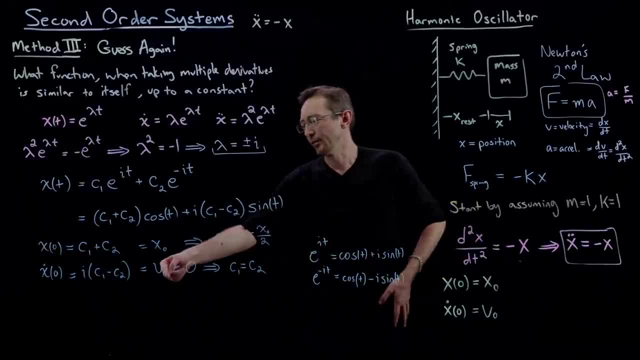 equals C 2. so C 1 equals C 2 equals X equals C 2 equals C 2 equals X. naught over 2. you could definitely solve naught over 2. you could definitely solve naught over 2. you could definitely solve this for a nonzero velocity. I just don't. this for a nonzero velocity. I just don't this for a nonzero velocity. I just don't want to do it on the spot right now. that want to do it on the spot right now. that want to do it on the spot right now. that might be a good homework problem is kind. 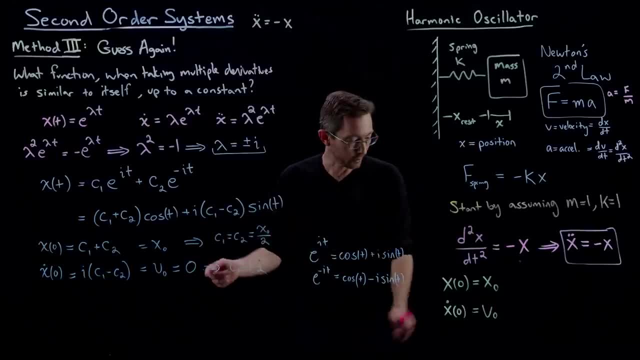 might be a good homework problem is kind might be a good homework problem is kind of work out the complex analysis. if this of work out the complex analysis, if this of work out the complex analysis, if this is a non zero V naught but for initial is a non zero V naught but for initial. 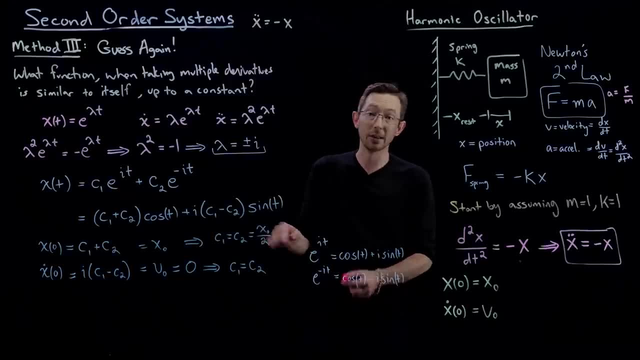 is a non zero V naught but for initial velocity equal to zero, these constants. velocity equal to zero, these constants, velocity equal to zero. these constants have to equal each other and they both have to equal each other, and they both have to equal each other and they both equal. X naught over over 2, and so that 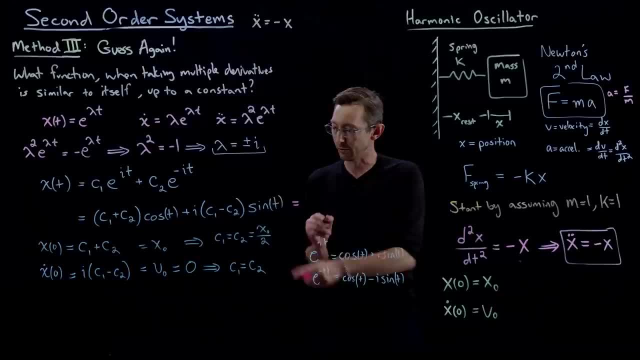 equal X naught over over 2 and so that equal X naught over over 2, and so that literally means that the solution again literally means that the solution again literally means that the solution again is equal to X naught cosine T- good okay. is equal to X naught cosine T- good okay. 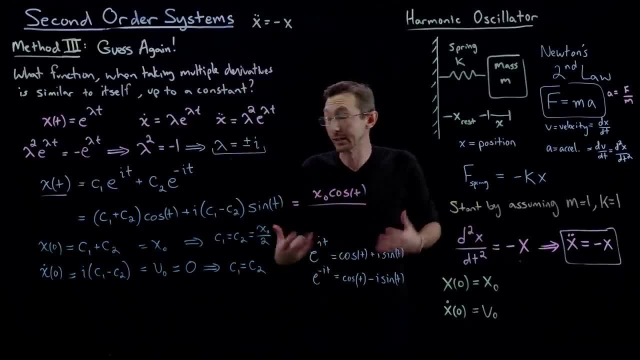 is equal to X naught cosine T. good, okay, so that again is a third way of. so that again is a third way of. so that again is a third way of confirming our intuition, that this thing confirming our intuition, that this thing confirming our intuition, that this thing is going to be built up of sines and is going to be built up of sines and is going to be built up of sines and cosines, and that these constants are cosines and that these constants are cosines, and that these constants are going to be used to get my initial, going to be used to get my initial. 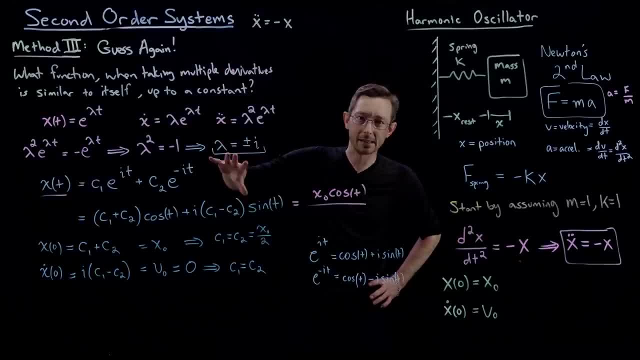 going to be used to get my initial condition and initial velocity. okay, I'll condition and initial velocity. okay, I'll condition and initial velocity. okay, I'll erase this and show up the fourth method. erase this and show up the fourth method. erase this and show up the fourth method, and we'll just briefly talk through that. 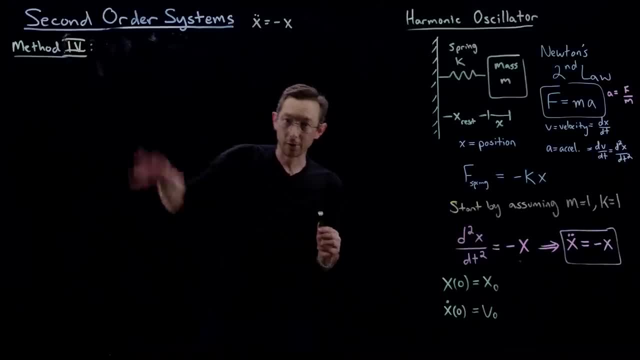 and we'll just briefly talk through that. and we'll just briefly talk through that. okay, so the fourth method. I'm just gonna. okay, so the fourth method, I'm just gonna. okay, so the fourth method. I'm just gonna write this down. I'm actually not going. write this down. I'm actually not going write this down. I'm actually not going to solve it using this method, but this is to solve it using this method. but this is to solve it using this method. but this is going to be the basis of a lot of the. 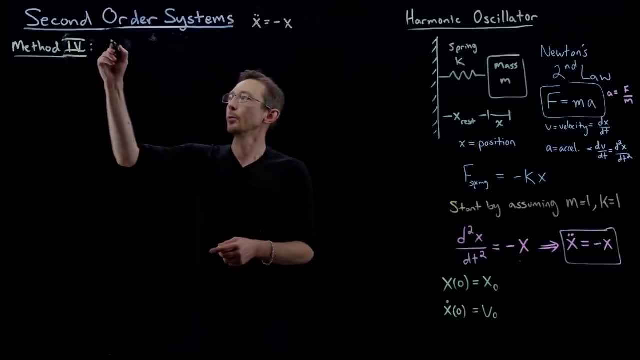 going to be the basis of a lot of the going to be the basis of a lot of the future lectures is method 4 is what future lectures is. method 4 is what future lectures is. method 4 is what we're going to do, is we're going to. 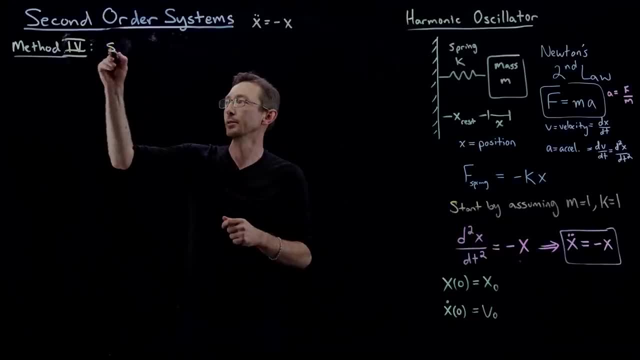 we're going to do, is we're going to we're going to do, is we're going to introduce a new variable. where this is, introduce a new variable. where this is, introduce a new variable where this is called suspending the variables, so called suspending the variables. so 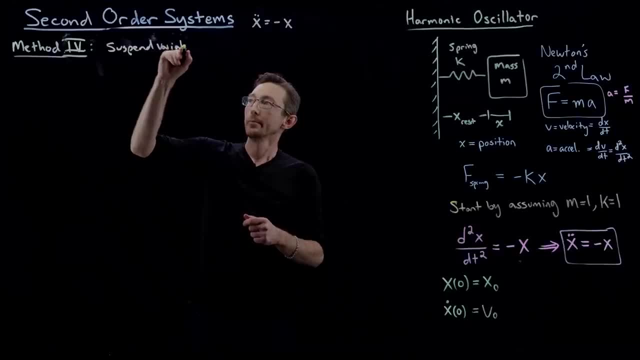 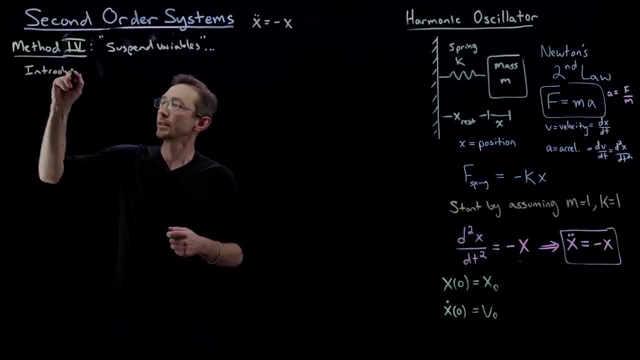 called suspending the variables. so suspend variables, essentially what that suspend variables, essentially what that suspend variables. essentially. what that means is that we introduce a new means, is that we introduce a new means, is that we introduce a new variable V, introduce a new variable V, variable V. introduce a new variable V. 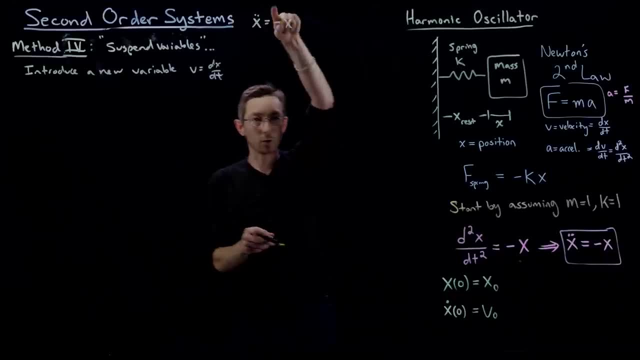 variable V. introduce a new variable: V equals DX- DT and I'm going to turn equals DX- DT and I'm going to turn equals DX- DT and I'm going to turn this second order linear differential, this second order linear differential, this second order linear differential equation into a system of first-order. 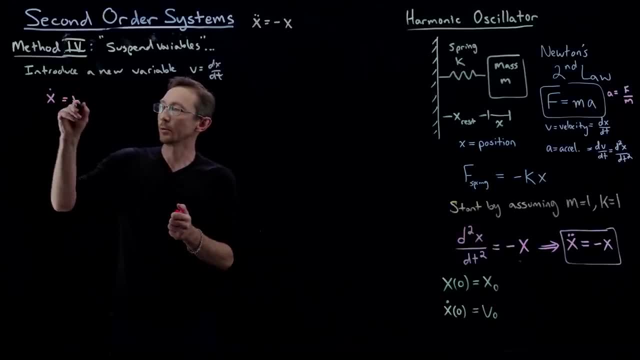 equation into a system of first-order equation, into a system of first-order differential equations. so I'm going to differential equations, so I'm going to differential equations. so I'm going to say X dot equals V, and now V dot equals. say X dot equals V, and now V dot equals. 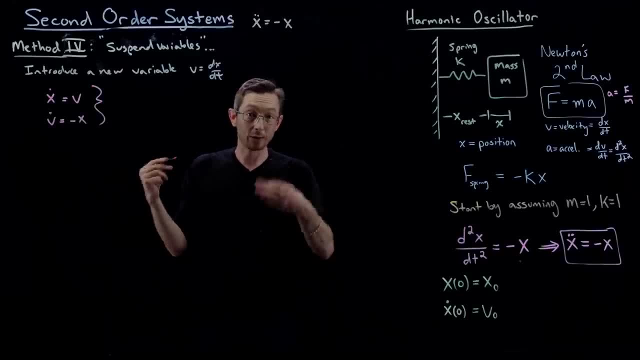 say X dot equals V, and now V dot equals minus X, and this allows me to write this minus X, and this allows me to write this minus X, and this allows me to write this as a matrix system of differential, as a matrix system of differential, as a matrix system of differential equations. so now I can have a vector X. 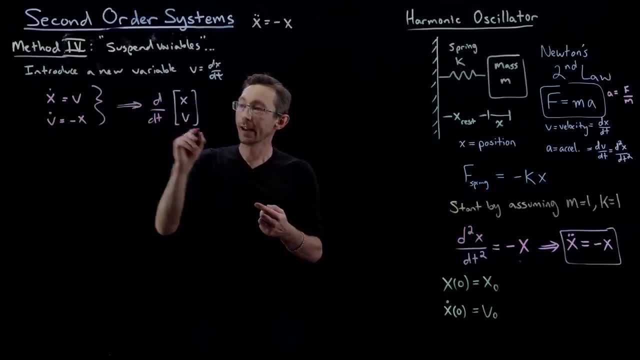 equations. so now I can have a vector X equations. so now I can have a vector X and V and DDT of this vector is going to and DDT of this vector is going to be a matrix times that state X and V, so DDT be a matrix times that state X and V, so DDT. 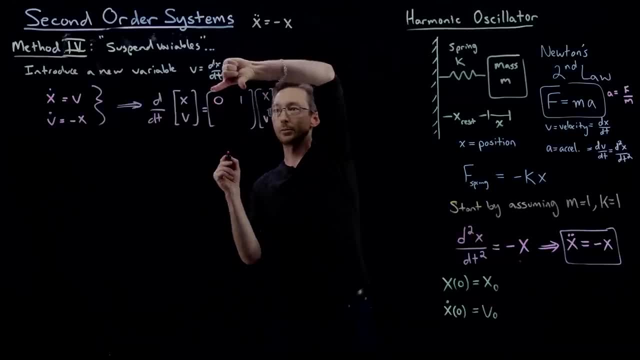 be a matrix. times that state X and V. so DDT of X is V, so that's 0. 1 that gives of X is V, so that's 0. 1 that gives of X is V, so that's 0. 1 that gives me X dot equals V. DDT of V is minus X, so I. me X dot equals V. DDT of V is minus X. so I me X dot equals V. DDT of V is minus X. so I put a minus 1 here and 0 there, that is. put a minus 1 here and 0 there, that is. 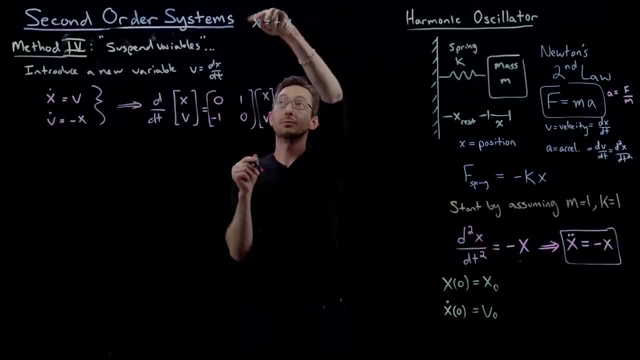 put a minus 1 here and 0 there. that is that equation. and now I went from a that equation and now I went from a that equation and now I went from a second-order system meaning I have second-order system, meaning I have second-order system, meaning I have second derivatives, because Newton's 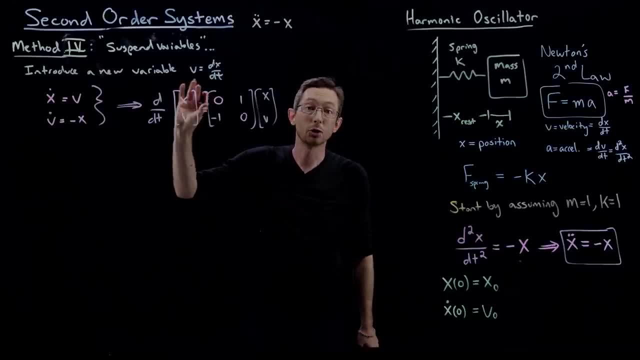 second derivatives. because Newton's second derivatives, because Newton's second law has second derivatives. now I second law has second derivatives. now I second law has second derivatives. now I have a system of two first-order systems, have a system of two first-order systems, have a system of two first-order systems. these are only first derivatives. so this: 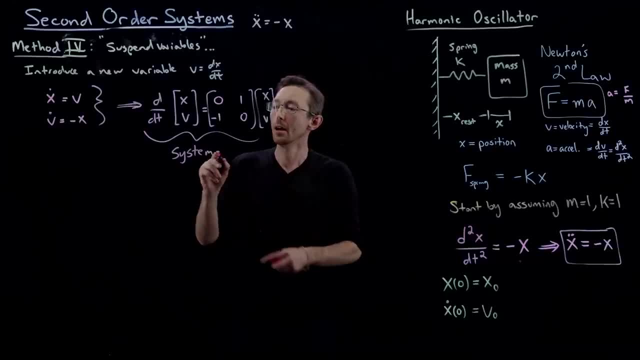 these are only first derivatives. so this, these are only first derivatives. so this is a system kind of a matrix system of. is a system kind of a matrix system of. is a system kind of a matrix system of first-order ODEs and you can always do. 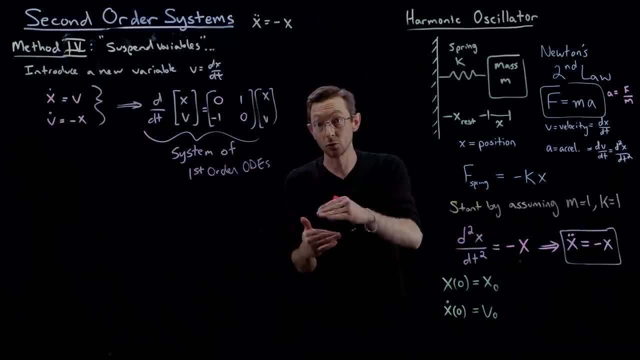 first-order ODEs and you can always do first-order ODEs and you can always do this if you have a second-order system. this, if you have a second-order system, this: if you have a second-order system- you can get as a system of two coupled. 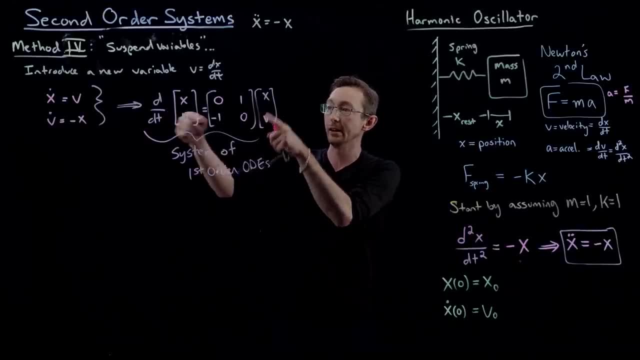 you can get as a system of two coupled. you can get as a system of two coupled first-order equations. they're coupled, first-order equations. they're coupled, first-order equations. they're coupled because X dot depends on V and V dot, because X dot depends on V and V dot. 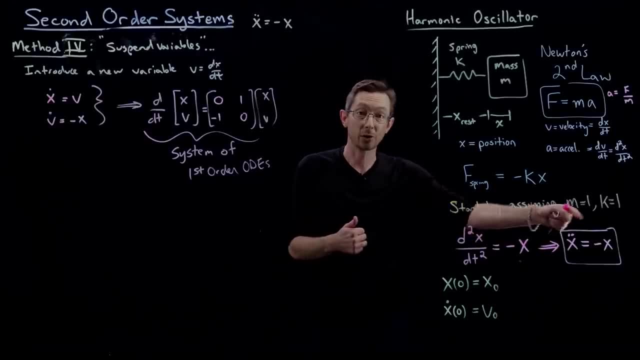 because X dot depends on V and V dot depends on on X. if I have a third depends on on X. if I have a third depends on on X. if I have a third derivative and X triple dot equals derivative and X triple dot equals derivative and X triple dot equals something. I could write this as a system. something. I could write this as a system, something I could write this as a system of three variables and so on, and so of three variables, and so on, and so of three variables and so on, and so forth. so I'll show you all of this in forth. so I'll show you all of this in. 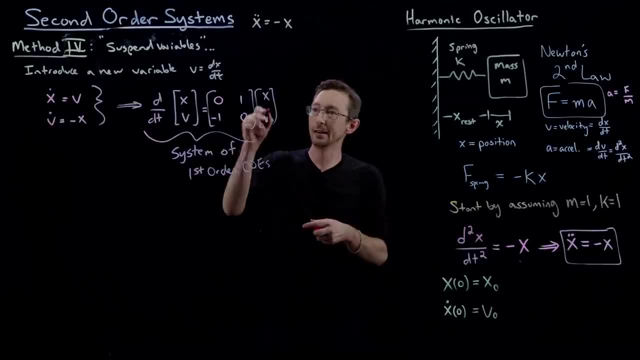 forth, so I'll show you all of this in the next lecture. but what's really neat the next lecture, but what's really neat the next lecture. but what's really neat here is that this vector now is the here. is that this vector now is the here is that this vector now is the state of my system that uniquely defines. 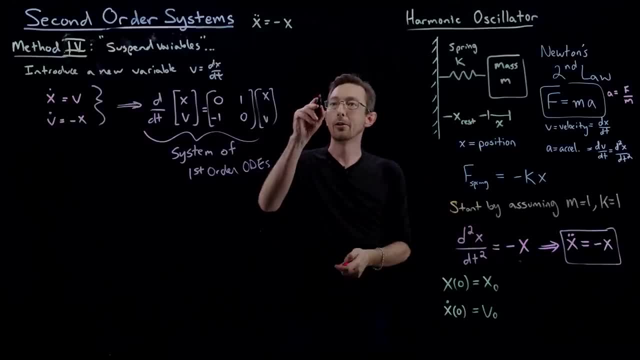 state of my system. that uniquely defines state of my system. that uniquely defines my system, the position and the velocity, my system, the position and the velocity, my system, the position and the velocity. and now I have, you know, an initial. and now I have, you know, an initial. 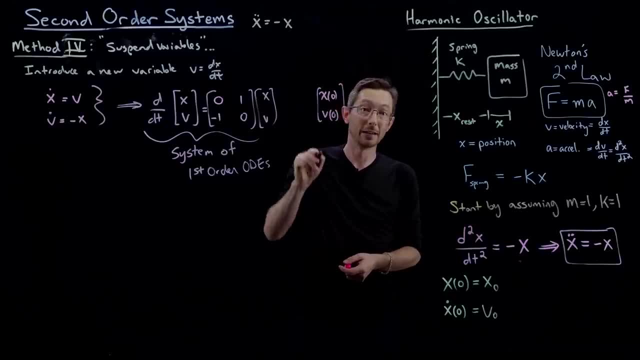 and now I have, you know, an initial condition: that again is a vector. you condition: that again is a vector. you condition: that again is a vector. you know X not, V not, and I'm going to show. know X not, V not, and I'm going to show. 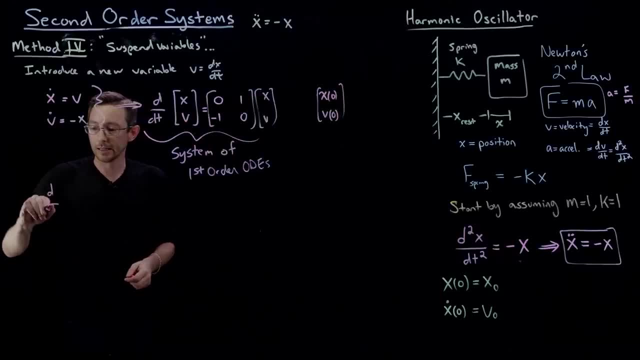 know X, not V, not, and I'm going to show you in in future lectures when you write you in in future lectures, when you write you in in future lectures, when you write this system DDT of- let's call it X and V. this system DDT of, let's call it X and V. 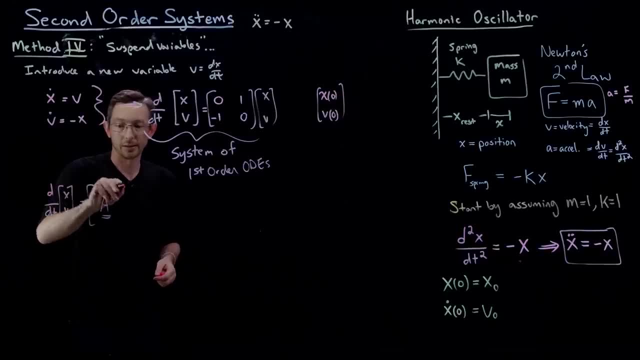 this system, DDT of- let's call it- X and V, equals this big a matrix. this is a equals this big a matrix. this is a equals this big a matrix. this is a 2x2 matrix: now times X and V, and I'm going. 2x2 matrix: now times X and V, and I'm going. 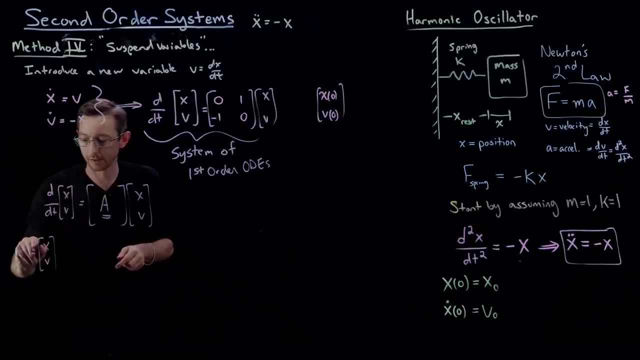 2x2 matrix, now times X and V, and I'm going to define this state X and V. we're to define this state X and V. we're to define this state X and V. we're going to call this like the bold, this. going to call this like the bold, this. going to call this like the bold. this underbar means it's a vector state. okay, underbar means it's a vector state. okay, underbar means it's a vector state. okay, that that means this, the state with two. that that means this, the state with two. 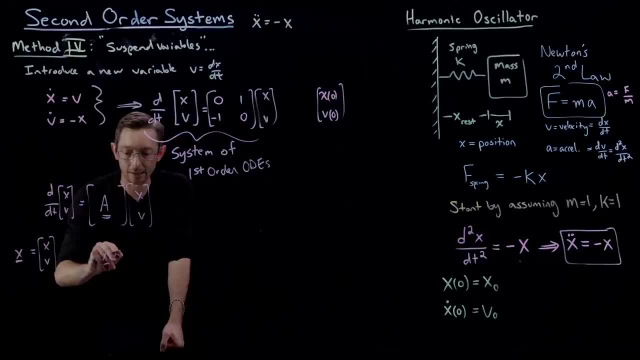 that that means this: the state with two components. we're going to see that X dot components. we're going to see that X dot components. we're going to see that X dot equals matrix a times X has a solution. equals matrix a times X has a solution. 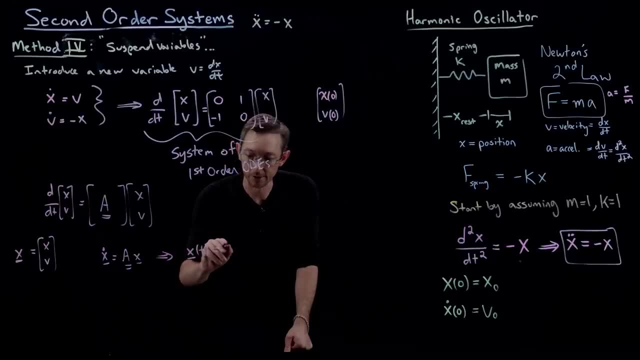 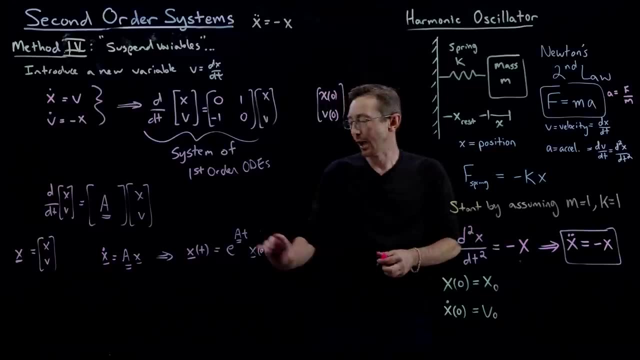 equals matrix a times X, has a solution which is X of T. equals the matrix which is X of T equals the matrix which is X of T. equals the matrix exponential e to the a- T times my vector exponential e to the a- T times my vector exponential e to the a- T times my vector of initial conditions: X at times 0. so of initial conditions X at times 0. so of initial conditions X at times 0. so I'm going to show you all of this in the. I'm going to show you all of this in the. I'm going to show you all of this in the future lectures. this is how we saw. 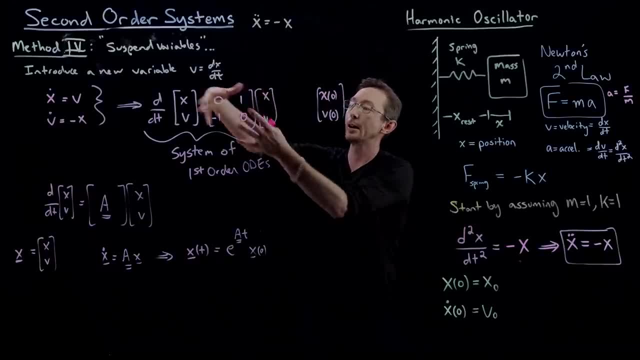 future lectures. this is how we saw future lectures. this is how we saw really big systems of equations, or really big systems of equations, or really big systems of equations, or really high order systems is by writing really high order systems, is by writing really high order systems, is by writing them in this matrix system of equations. 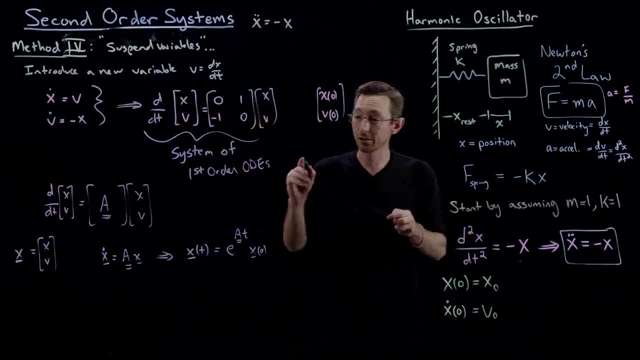 them in this matrix system of equations, them in this matrix system of equations, way and teaser those lambdas that I way and teaser those lambdas that I way and teaser those lambdas that I showed you, those lambdas that equal. showed you those lambdas that equal. 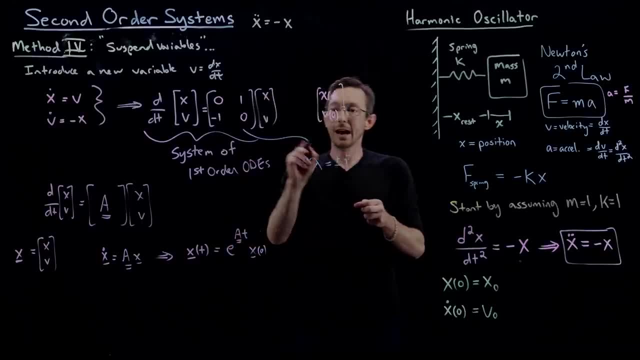 showed you those lambdas that equal plus and minus I. those are the eigen plus and minus I. those are the eigen plus and minus I. those are the eigen values, the eigen values of the same values, the eigen values of the same values, the eigen values of the same matrix. okay, so the eigen values of this. 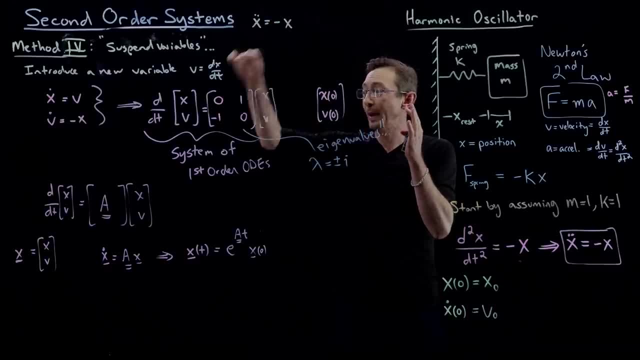 matrix. okay, so the eigen values of this matrix. okay, so the eigen values of this a matrix. when you, when you suspend a matrix, when you, when you suspend a matrix, when you, when you suspend variables and write this as a system of variables and write this as a system of. 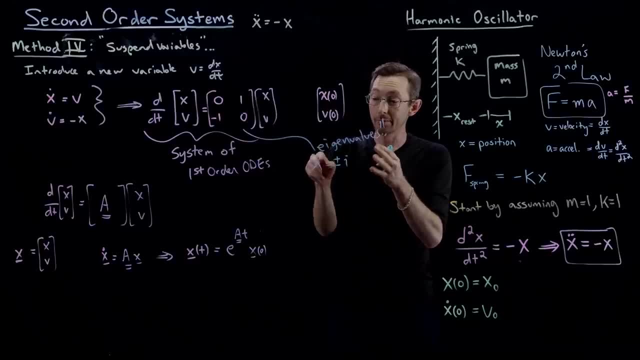 variables and write this as a system of first-order equations: the eigen values, first-order equations. the eigen values, first-order equations. the eigen values of that a matrix are the lambdas. the of that a matrix are the lambdas. the of that a matrix are the lambdas, the kind of e to the lambdas that you would. kind of e to the lambdas that you would kind of e to the lambdas that you would use to solve the system. so that's going use to solve the system. so that's going use to solve the system. so that's going to be a deep connection. that's how we're. 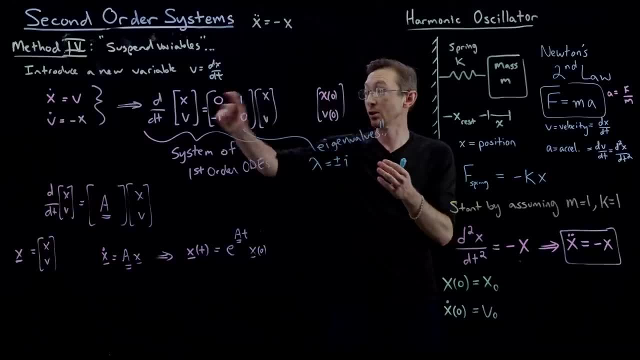 to be a deep connection. that's how we're to be a deep connection. that's how we're actually going to derive the eigen value actually going to derive the eigen value actually going to derive the eigen value and eigen vector equation is to solve, and eigen vector equation is to solve. 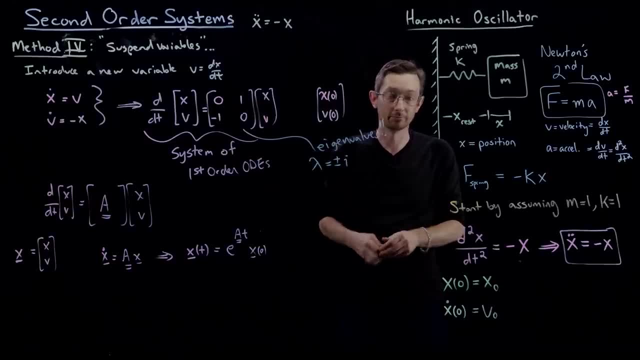 and eigen vector equation is to solve these equations and that's all coming up, these equations, and that's all coming up, these equations, and that's all coming up soon, thank you.